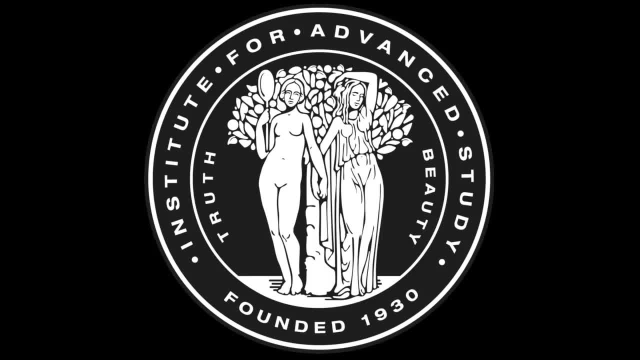 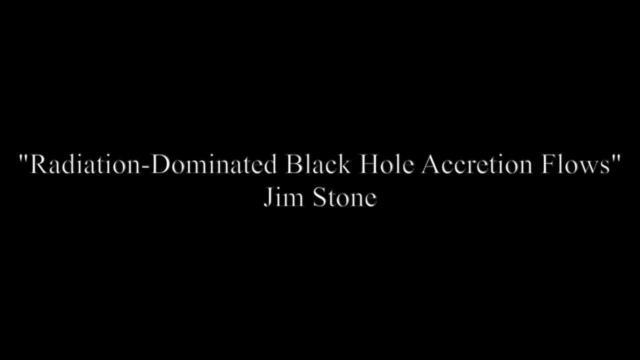 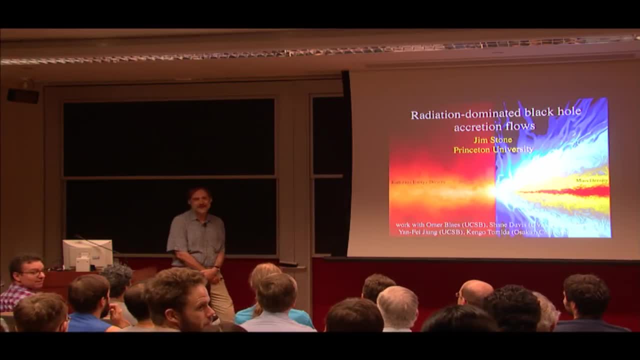 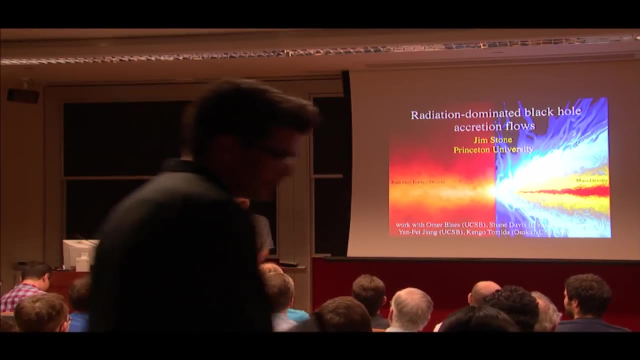 Thank you, David. It's always nice to give a talk in front of the hometown crowd, hopefully a friendly crowd, but after that outburst from Mr Lupton, I'm not sure. Dr Lupton, Dr Lupton. 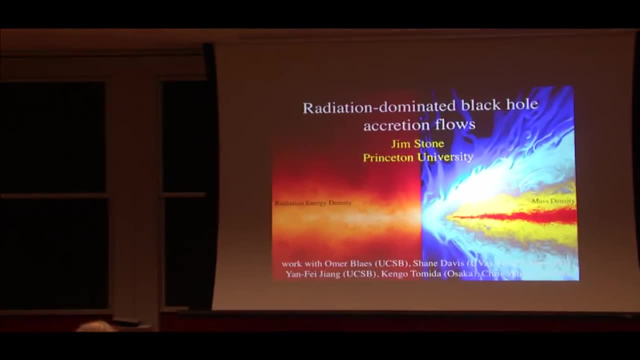 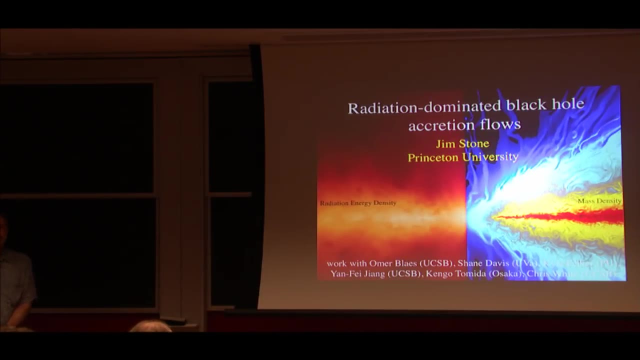 And so it starts. So when I was first asked to give this talk, I thought, well, I've just given a talk at the Institute. Really we should let somebody else give the talk. But then I look back in my archive of presentations and realize it's been more than six years since I gave a talk. 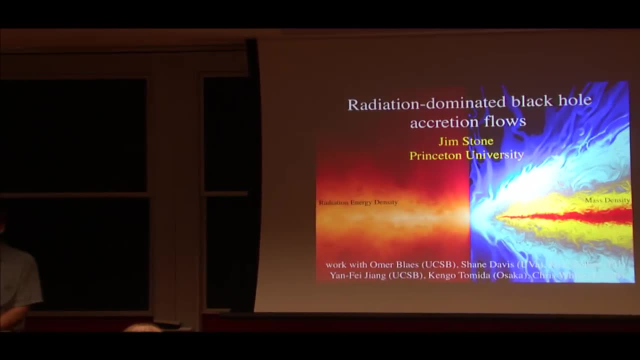 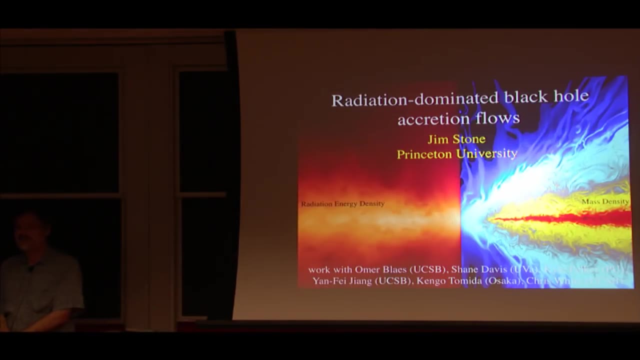 here. Time flies when you're having fun. But then I also realized that the subject of the talk I gave six years ago was the same subject as the talk today. I may be a little bit worried, but I assure you that there are lots of new results here. 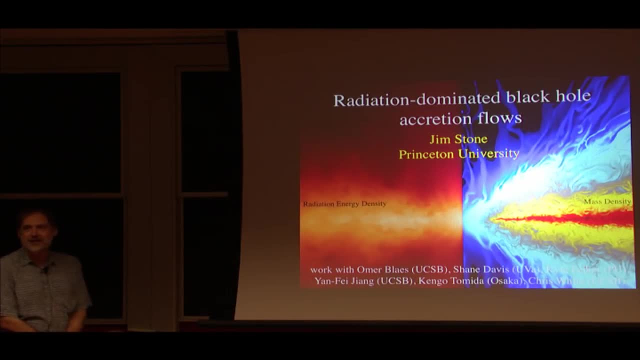 You know, one could say that, well, maybe we're not very imaginative, We keep working on the same things. But I would also say this is a really hard problem, It's a very important problem And it's worth spending some time to get right. And, I think, the ability to do 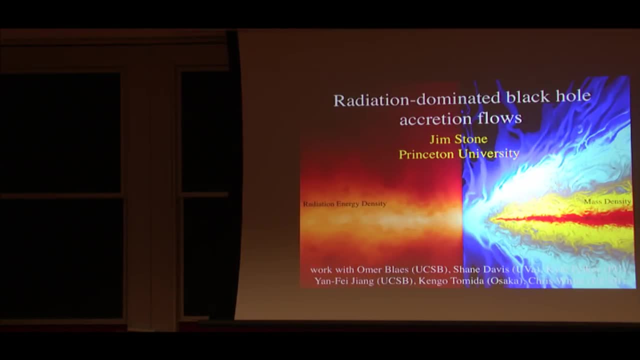 ab initio calculations with radiation and MHD is a new capability. that's going to be that not only our group but other groups are doing. It's very, very exciting- So it's been long enough- that my collaborator list is continuing to grow And people like 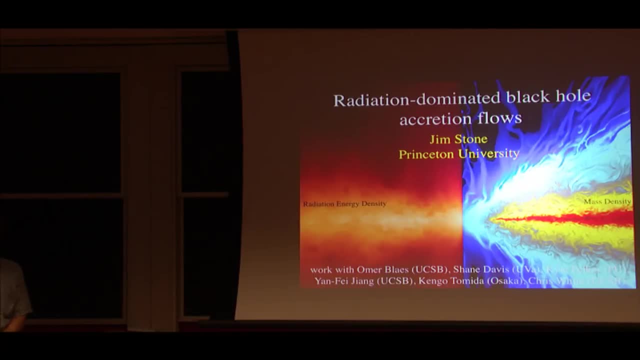 Yanfei Zhang, who was a student at the time I gave my last talk, is now moving to Beijing University this next coming year as a professor. Shane Davis was a member here back then. He's now a professor at the University of Virginia. Kengo Tomito had just been finished a visit. 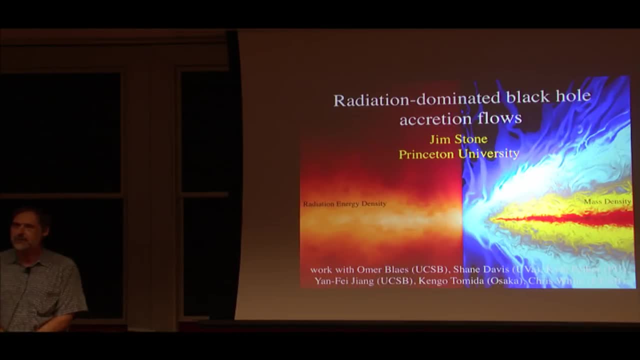 as a visiting research student collaborator. He's now a professor at Osaka. Chris White has done his thesis and graduated. I point out that my collaborators involve a lot of students and postdocs who have been here over the years And they've made very, very. 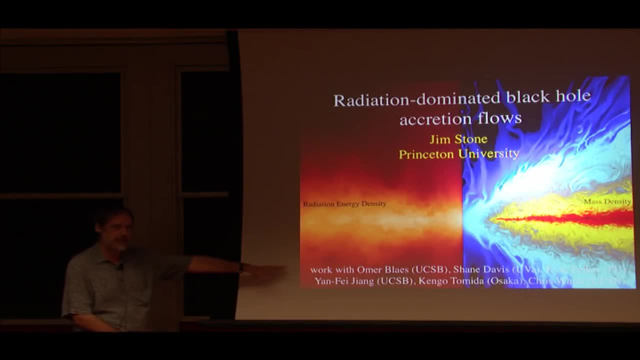 fundamental contributions. especially Yanfei has done an amazing job with this. I want to highlight his contribution. So the image in the background is a calculation that I'm going to try to explain to you what it means and how we did it. So why are we interested? I'm going to start with a quick motivation. I'll describe briefly. 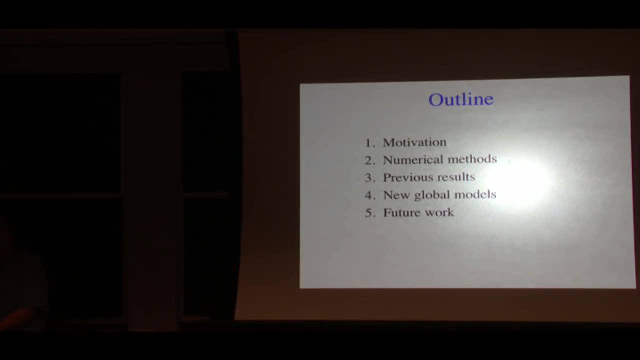 some numerical methods. previous results Now I recognize. over the last six years I've given talks on this subject at lots of different places And I suspect there's grad students and postdocs here that have probably seen me give parts of these results to you And I. 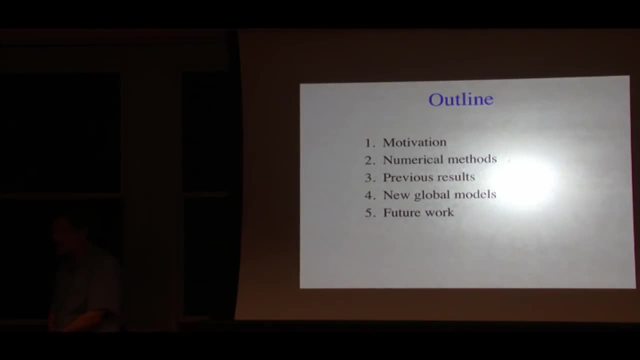 know you've probably seen me talk about these results before, But I promise there's lots of new results. I'm not going to spend too much time on the previous results, like we've talked about elsewhere, So bear with me. I'll mostly talk about some new global models. 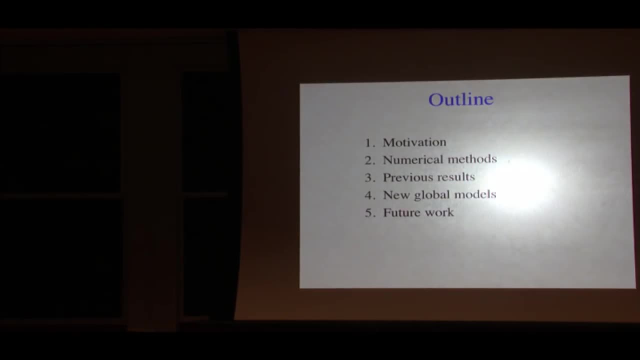 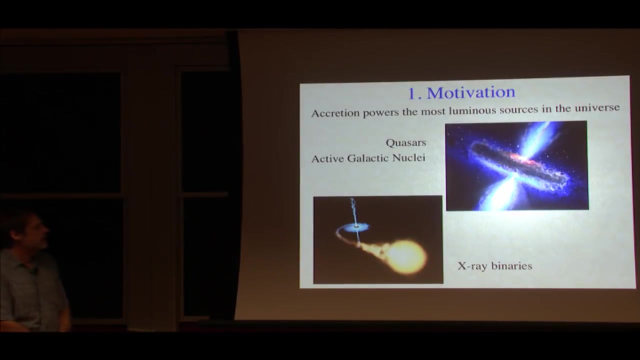 including some unpublished results on sub-ethnic accretion flows. So why do we want to study this problem? And the answer is very, very simple: Accretion powers, all the most luminous sources, Quasars and active galaxies, when the creating source 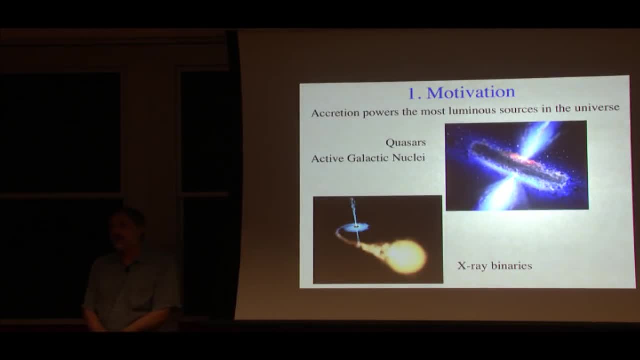 is a supermassive black hole, X-ray binaries when it's a stellar mass black hole. So if we want to understand these sources, we need to understand more about the problem And then we can start to think about the problem and how we can use these models and other. 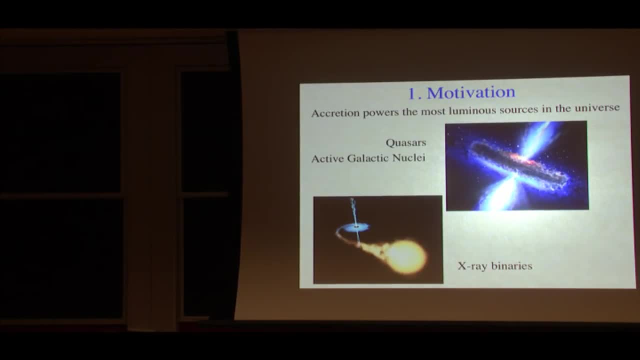 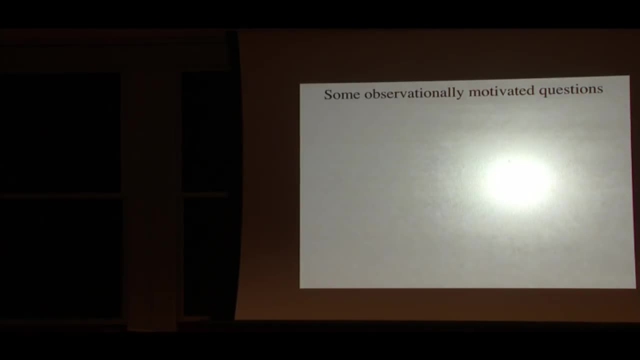 to understand the accretion process itself And we can zoom in a little bit more on a little more specific questions. There's a couple of questions that I personally think have been highly motivating for our project. Some amazing results in the last decade or so. 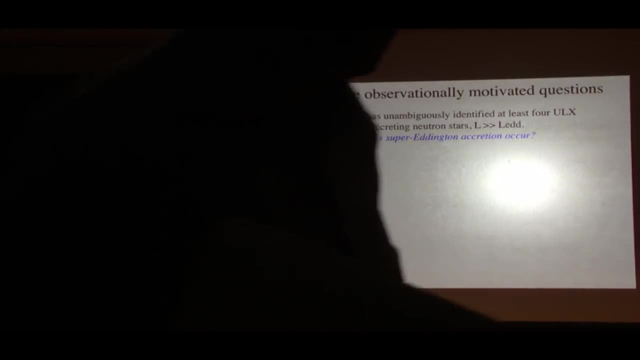 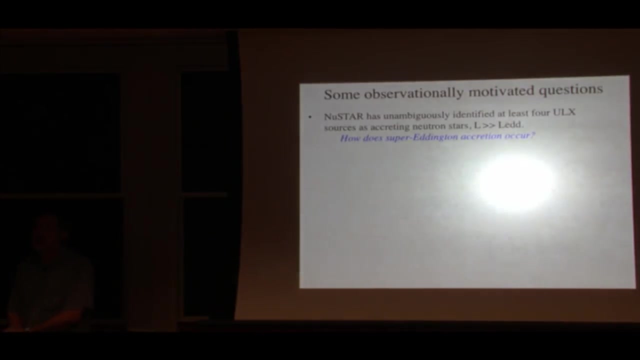 For example, the NuSTAR mission has unambiguously identified at least four ultra-luminous X-ray sources as being accreting neutron stars. That means that their luminosity is hundreds of times the Eddington luminosity, And that's remarkable. 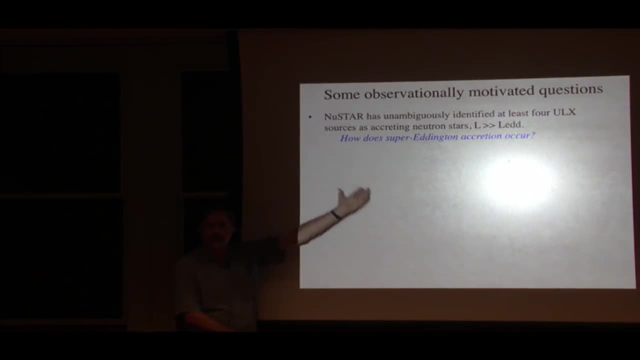 These sources were originally thought to be intermediate mass black holes, because how could you have super Eddington accretion? Well, now we know for sure super Eddington accretion is occurring in these systems. So how does that work? That's a very important question. 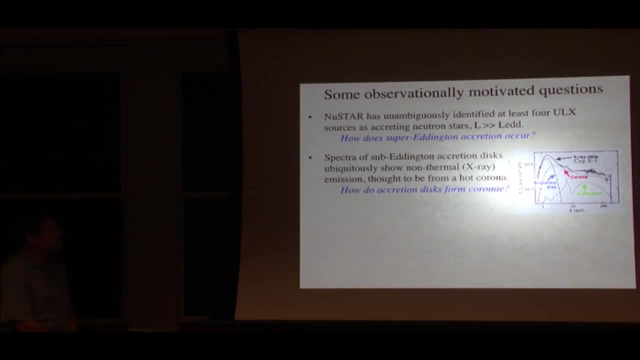 A long standing question for decades is that spectra of sub-Eddington accretion, whether it be stellar mass or supermassive black holes, show non-thermal X-ray emission thought to be from a very hot corona. So how do you make that corona? 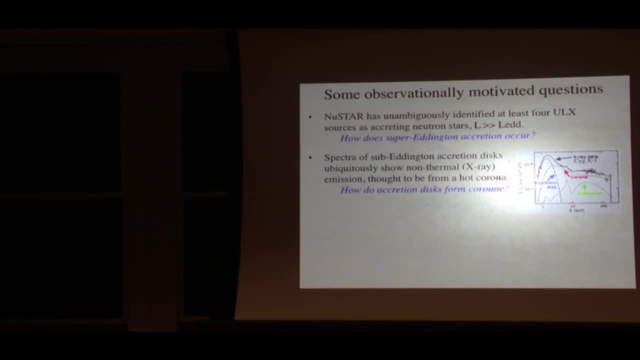 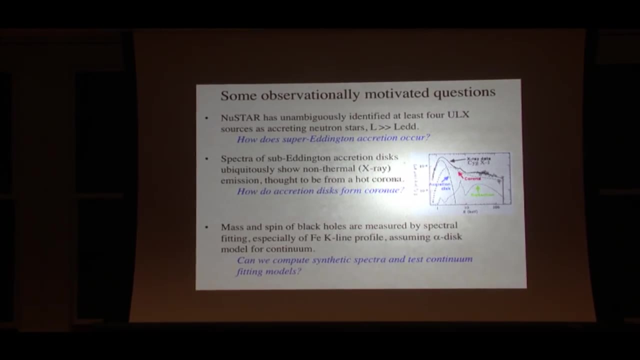 There's dozens of papers that describe mechanisms for making corona. Can we see unambiguously the formation from corona, from these accretion flows? And then, finally, we want to measure the properties of black holes, And one way you do that is through spectral fitting. 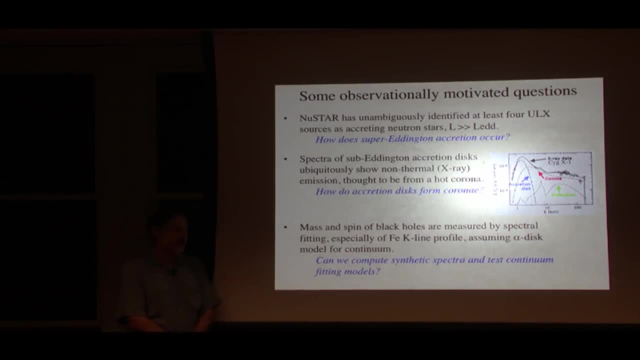 especially of the red shifting of the iron k-line profile. But to get the line profile you have to subtract off the continuum, And the continuum comes from a simple alpha disk model And that's subject to question is whether that's really accurate. 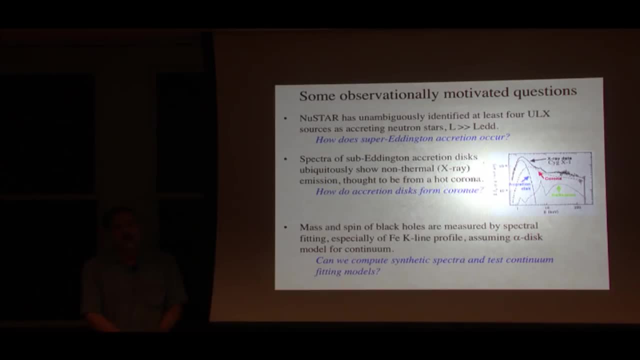 And if it's not accurate, that could affect your measurement of spin and mass And mass of the black hole. So can we calculate ab initio synthetic spectra that we could use to calibrate whether or not existing spectral fitting models are really accurate? 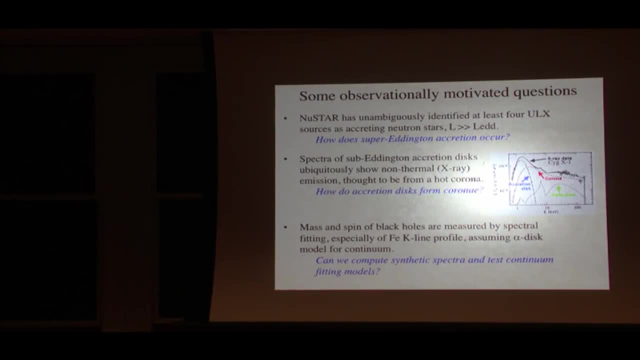 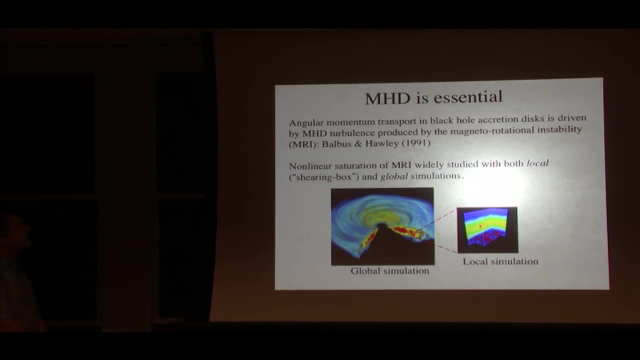 and we're really measuring the spins of black holes accurately. That's a very important question, a fundamental question: just understanding properties of black holes. So, if we want to do these calculations, what's required? Well, the first thing we have to do, 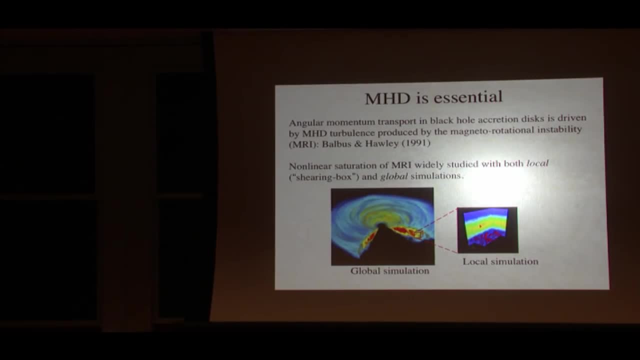 is include magnetohydrodynamics, MHD. That's because for the last 25 years, if you're in this department, you know for sure all about the magnetorotational instability That the accretion process itself is driven by MHD processes. 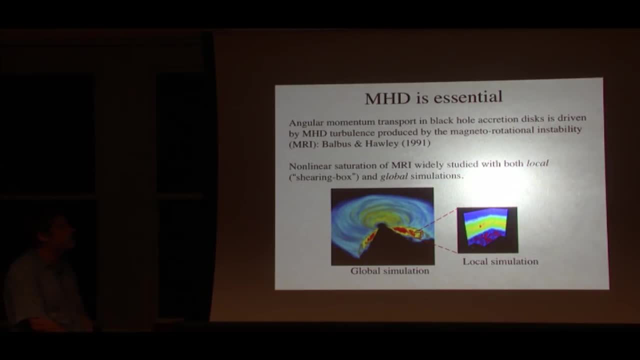 There's a linear instability in rotationally supported flows that produces turbulence. The properties of that turbulence has been understood through simulation, And so for 25 years we've been doing both global simulations incorporating the entire disk, or local shearing box calculations to focus in on the physics of MRI turbulence. 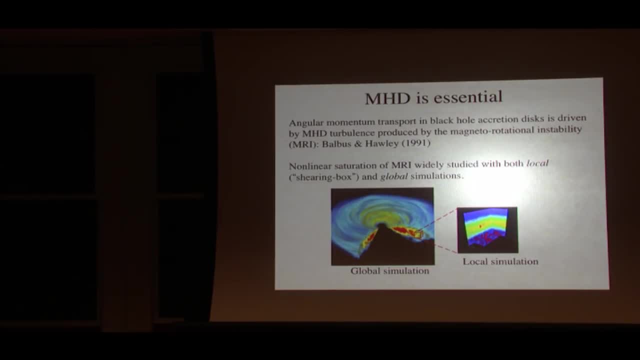 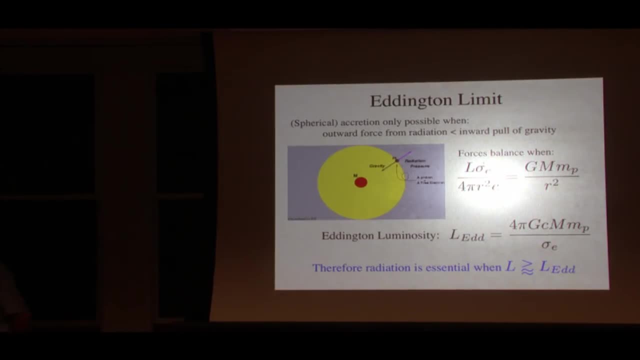 And so we need to include that physics if you're going to have a first principles model of these accretion flows. And then I've mentioned this Eddington limit a couple of times, So just to remind students, for example, what that really 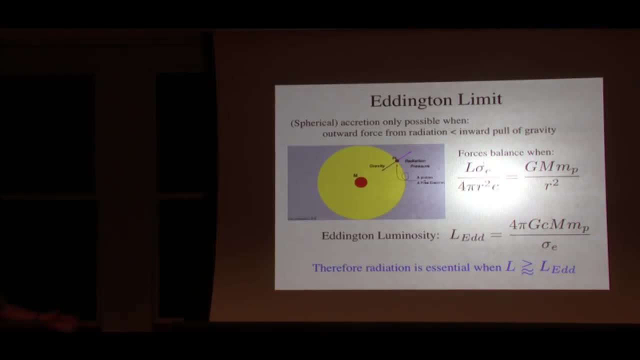 means in a spherically symmetric, one dimensional picture of accretion. then it can only happen when the radiation force which is trying to push the plasma away is smaller than the inward pull of gravity, And so it's very simple just to equate those two forces. 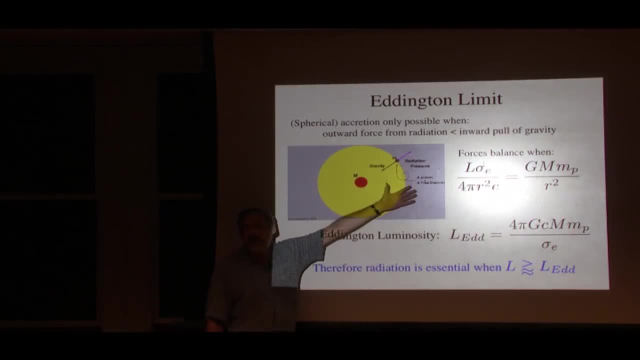 The radiation force is just the flux times, the electron scattering opacity, Because for a fully ionized plasma most of the opacity is coming from scattering off of electrons. So most of the radiation force is associated with that physics. And then, of course, far away from the black hole, 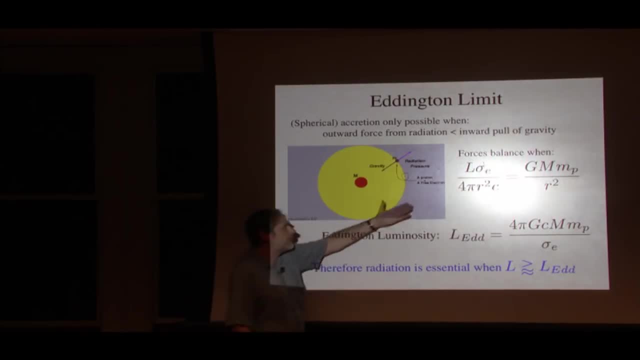 you can just use the Newtonian form for gravity with the mass of the proton here, because it dominates the mass budget of the plasma. It's a little funny because it seems like you're pushing on the electrons and pulling on the protons, But in fact they're tightly coupled. 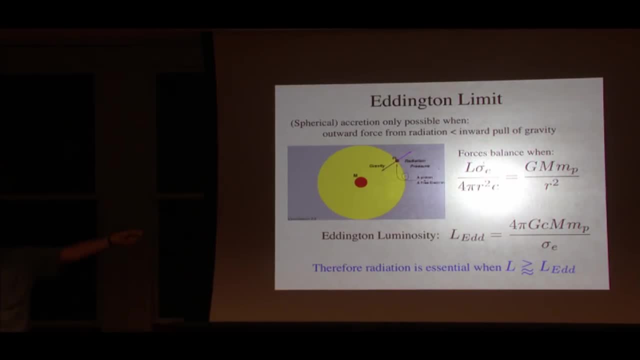 because electrostatic forces between them mean that if you push the electrons out, they drag protons along. So just equating those two it gives you the Eddington luminosity, The luminosity for a one-dimensional spherical flow. accretion would be halted. 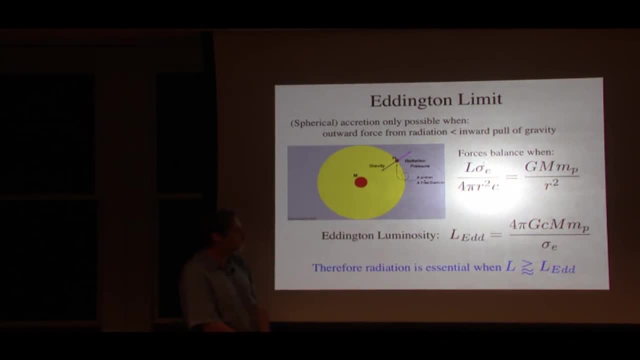 And it's just linearly proportional on the central mass of the object. So clearly we also need to include radiation if we're going to study flows anywhere near this Eddington limit. It turns out, as I'll show you today, that even if you're an order of magnitude less than that, 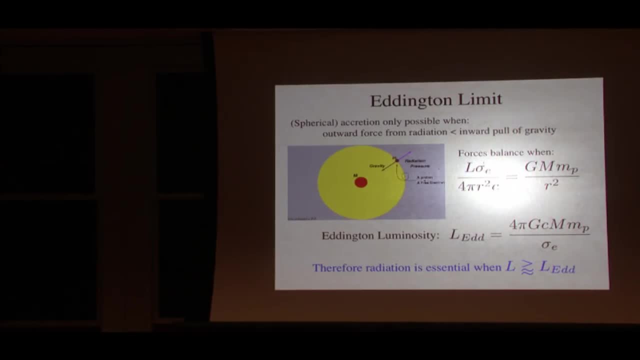 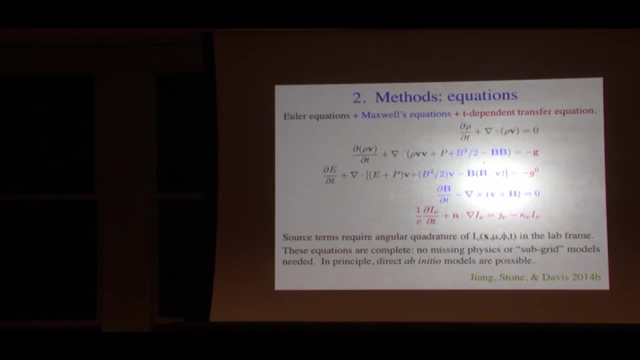 even two orders of magnitude less than that. radiation can play a very big role in the accretion physics, And so it's very important to include the radiation self-consistently along with the MHD and the dynamics. OK, So if we want to calculate these flows from first principles, 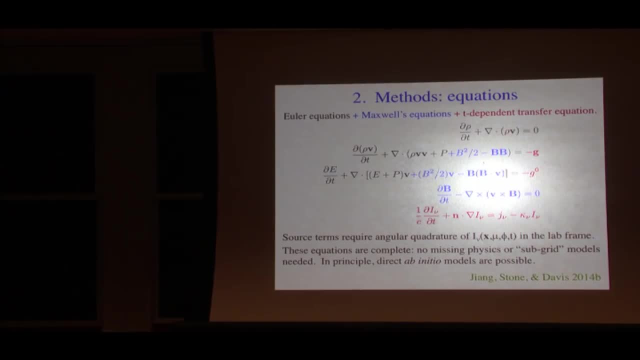 these are the equations we need to solve. This is the mathematical model we use to describe the flow. It's a highly collisional plasma, And so we can use the MHD approximation. So we have the regular equations of fluid dynamics, supplemented with the Maxwell's equations, the blue terms. 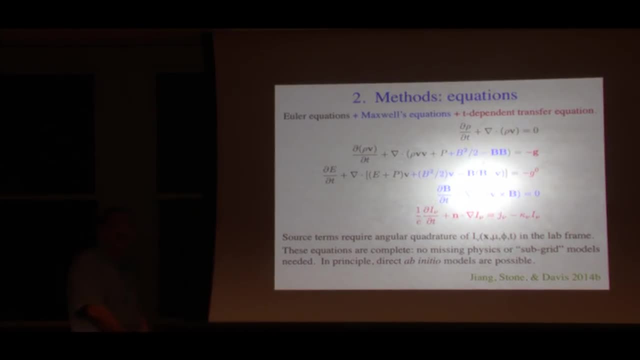 and equations to describe the evolution of the magnetic field, Because we're talking about temperatures that are 10 to the 5,, 10 to the 6,, 10 to the 7 Kelvin. the plasma is fully ionized, And so the ideal MHD approximation. 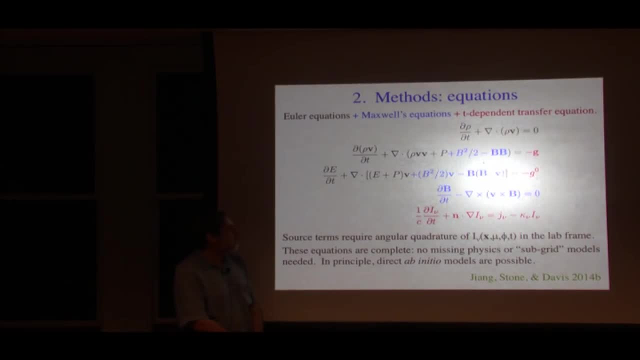 works extremely well for these models. So, in addition to the MHD equations, the blue and black, we also have to include radiation transport, which fundamentally is described by the radiation transfer equation. And then moments of the specific intensity. i give you the force acting on the fluid and the net heating. 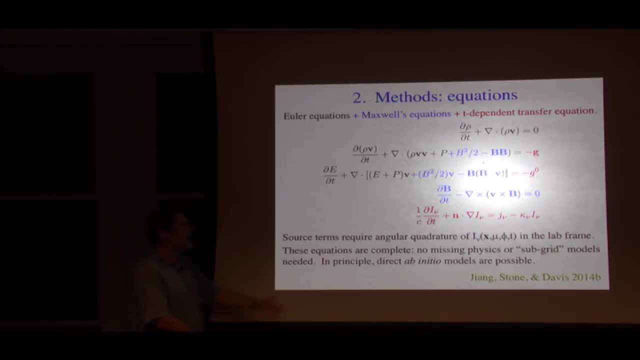 and cooling rate in the fluid. So if I know i, I can calculate these moments and calculate the forces and heating and cooling and the material radiation interaction terms. So it's a complicated set of hyperbolic partial differential equations which takes, I would say, 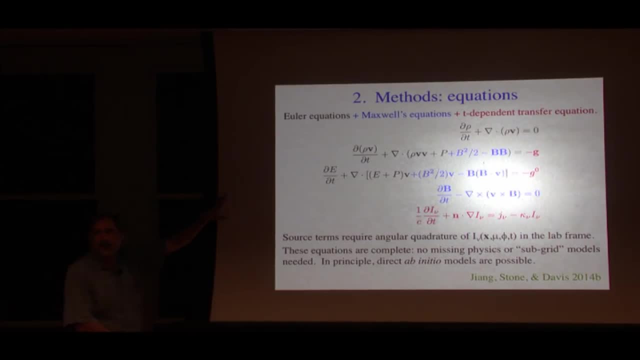 when I started graduate school, methods for hydrodynamics were pretty solid and mature and well used, And over my career, methods for MHD have become pretty solid, mature and well used. There's now half a dozen different algorithms for MHD and astrophysics that are very reliable and used. 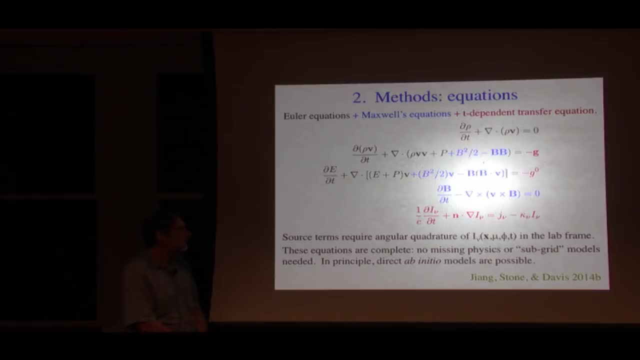 It's really radiation that's the frontier now. Incorporating from first principles radiation transport and including it directly in the dynamics is a challenging problem which I imagine is going to be another decade or so of people contributing before we're really going to understand exactly what's. 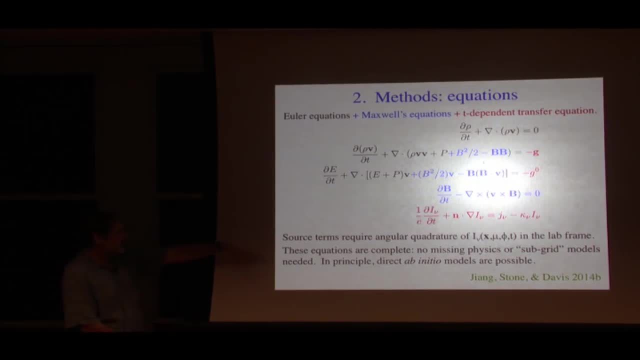 going on, But I would say, and I like to point out, that these equations are complete. There's no missing physics, no subgrid model that we have to put in, And many problems in astrophysics like, say, galaxy formation is the best example. 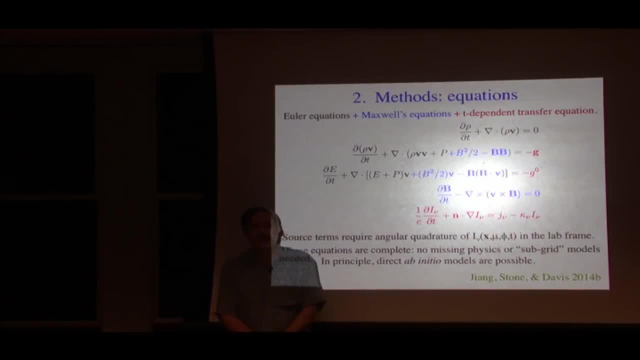 There's things going on at small scales we can't resolve, and so you have to add in subgrid models. No subgrid models here. If we can just solve these equations accurately, we should be able to understand the flows directly. And if solutions of these equations 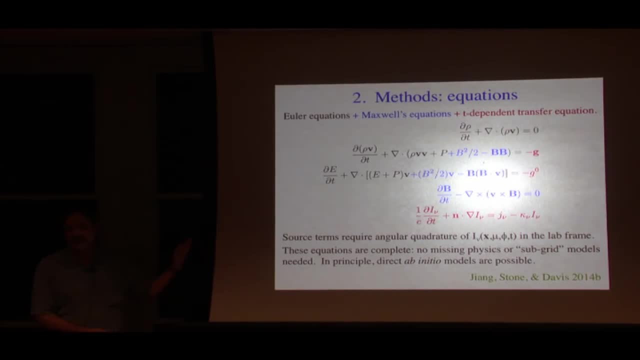 don't agree with observations, then we're missing something very fundamental in the physics. that's going to be very, very instructive. In that sense, the task is easy: Just solve these equations Well, you need to understand some of that. 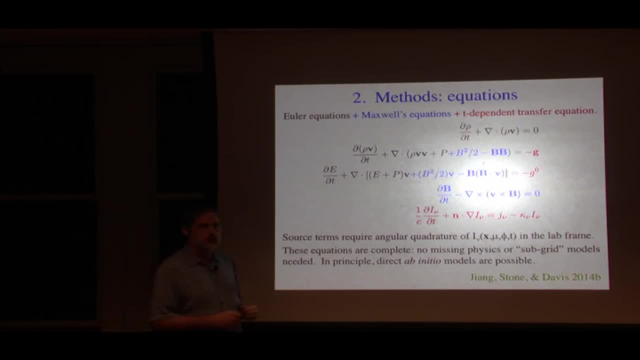 That's Well for these temperatures. it's pretty simple. It's mostly just electron scattering. You're absolutely right that farther out in the disk, where the gas gets cooler, the opacity gets complicated. So you're absolutely right that there. 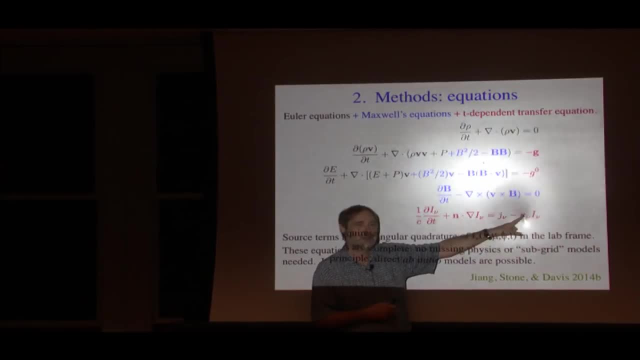 is an awful lot buried in this thing here, And you can get different solutions depending on what the opacity, But that's still classical physics that we understand. You can put in two-level atoms if you need to. You can put in approximations for treating. 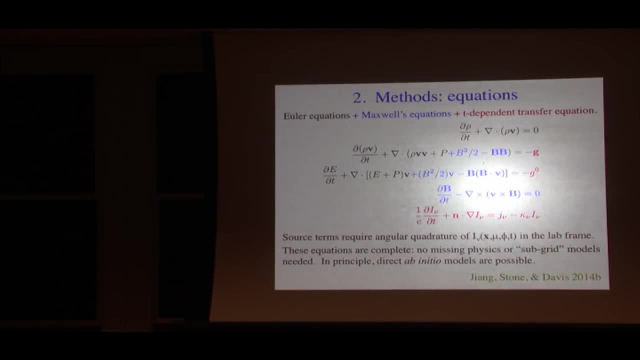 all those things, It's sort of not missing physics, It's just more complicated things to look at. Yes, Yes, We don't resolve it all the way down to the viscous scale across 10 orders of magnitude, But you resolve it over the inertial range. 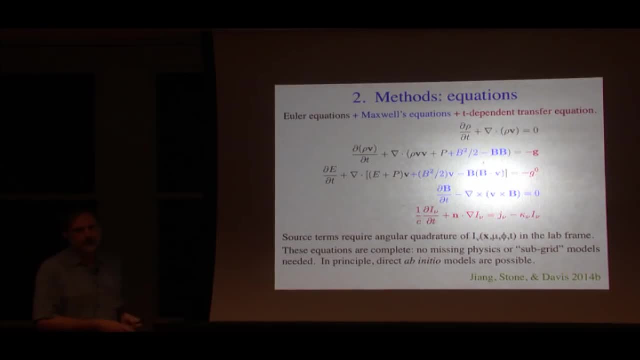 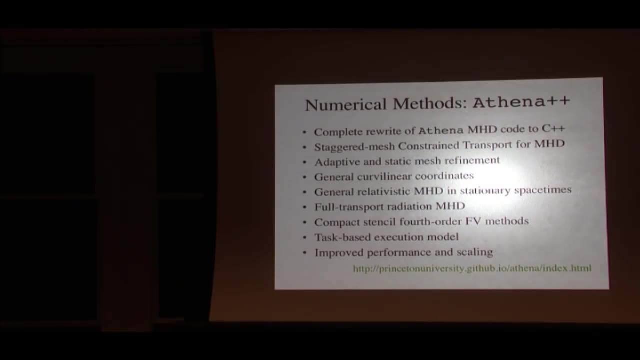 to be able to capture the driving scale and the cascade in the inertial range. OK, So we're going to need numerical methods to proceed, I mean, except in the simplest cases. analytic solutions for those equations are just not viable. And so one thing that's changed in the last six years. 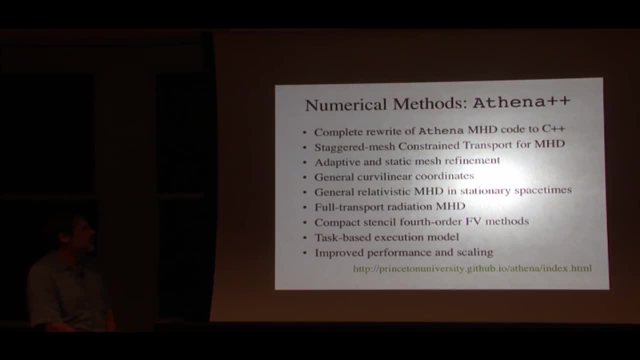 is a whole new code. That's a significant step forward, I would say So. Athena++ is a complete rewrite of the Athena code, mostly driven by the need to use general curvilinear coordinates to study these flows and to be able to have 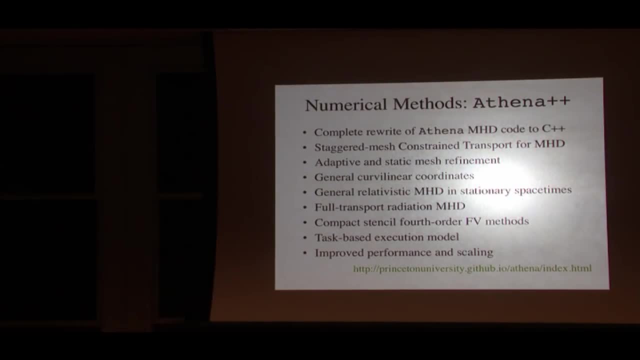 fully adaptive and static mesh refinement. That was the major driver in rewriting the old version of Athena was. to extend it to those capabilities was going to be way too much work. It was much easier just to start from scratch again And along the way Chris White added GRMHD. 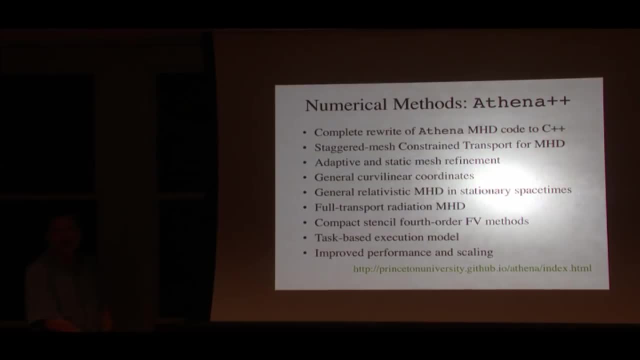 and stationary spacetimes. Yanfei's added this full transport radiation, which I'll talk about. Kyle Felker, who's here, is adding compact stencil, high order methods And there's various other features that are very, very important for making this code efficient. 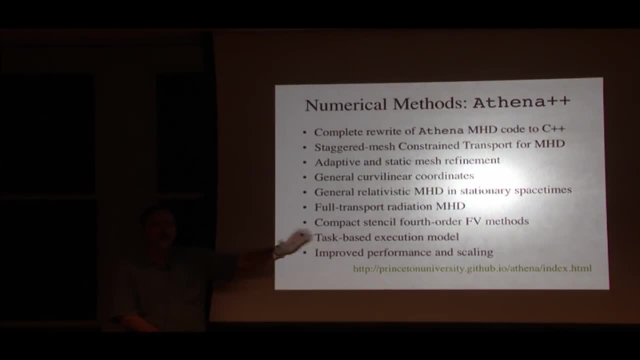 And the code's fully available. It's available on GitHub. It's freely. There's a public website. You can download the code directly from GitHub if you like and play with it and use it for any problem you might be interested in. 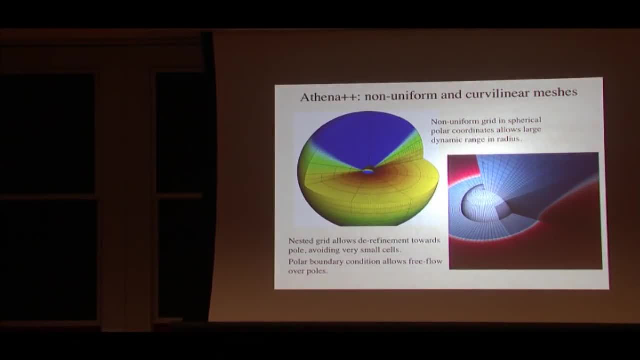 So I mentioned the static mesh. It's because we expect this rotationally supported flows to be sort of concentrated to the equatorial plane And we want to resolve the turbulence in the disk, And so we need fine resolution towards the midplane and less resolution towards the pole. 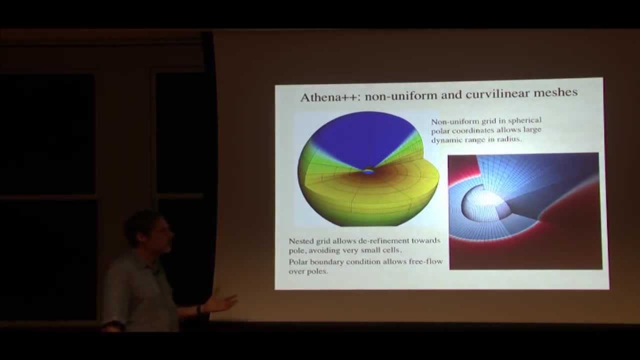 And so this curvilinear mesh can be used in spherical polar coordinates, which is well-suited for these kind of accretion geometries. And, moreover, this adaptive mesh can allow us to resolve the turbulence in the midplane, And that's an important feature to enable us to have. 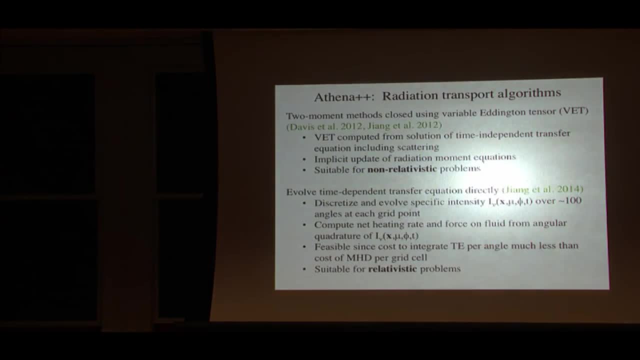 more accurate calculations. Most important is the radiation transport algorithms, And there's a lot here and I'm just going to brush over quickly. There's sort of two basic algorithms that are implemented in the code. One is using a two-moment closure. 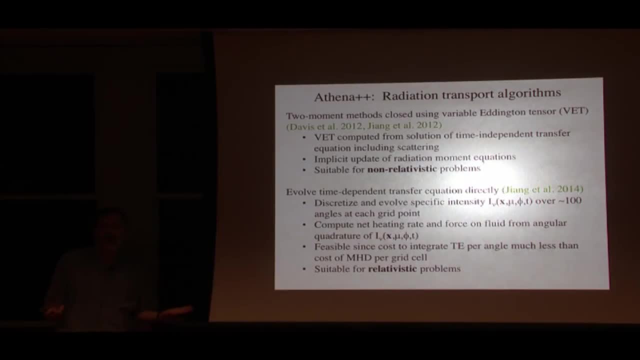 based on the variable Eddington tensor, where we solve the time-independent transfer equation to compute the geometry of the radiation field and compute the closure directly. It adopts an assumption, namely that the flow times are very, very long compared to the light crossing time. 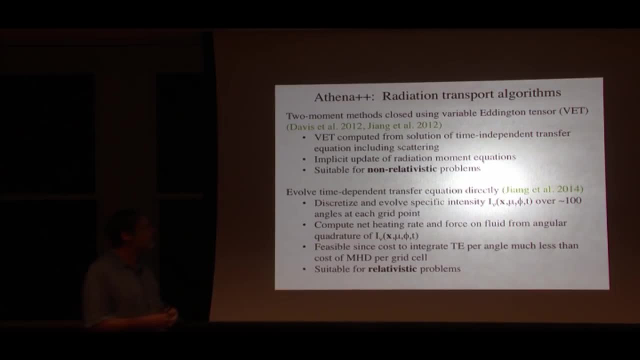 So we can use this non-time-dependent transfer equation. So it's only really suitable for non-relativistic problems. Today I'm going to be describing results that come from a fully time-dependent solution of the transfer equation. We just bite the bullet: solve the transfer equation. 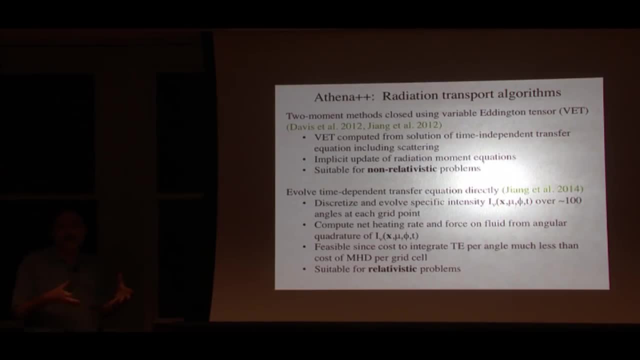 store the specific intensity And then we're going to take the specific intensity over up to 100 angles in every single grid point and evolve the specific intensity and time on every grid point, at every angle, and then compute moments of it to compute the net cooling rate. 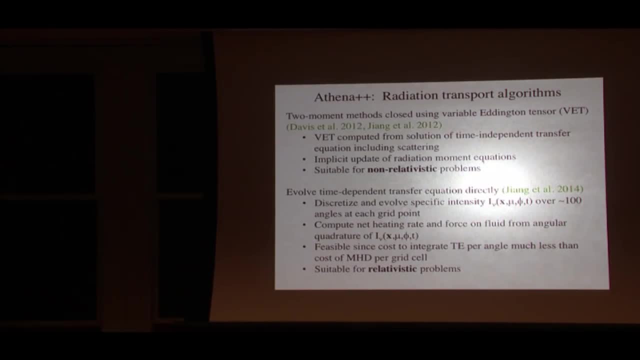 and the force in the fluid. It's expensive, but the MHD is expensive And computers are getting very, very fast And this is really the only way to go for a full sort of ab initio approach. There are approximations you can adopt in these closure problems. 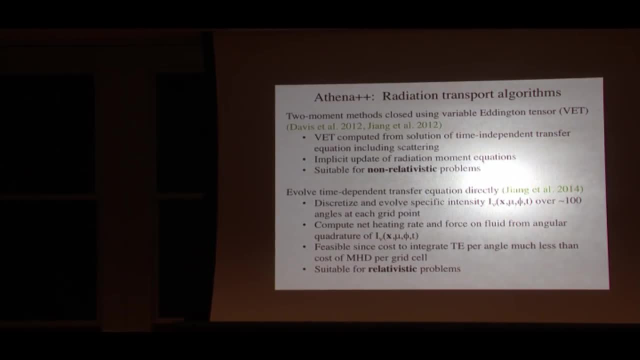 but they have issues, So I'll sort of mention that in a minute. So most of what I'm going to say today comes from this time-dependent transfer solver. And so how do we know We build this complicated code? It takes us half a dozen years to build. 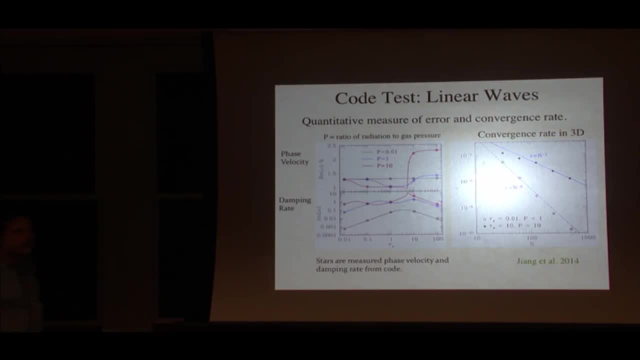 How do we know it's right? Well, actually known solutions to the equations of radiation MHD are hard to find. There's very few, And so we've done our best to try to find solutions. One solution comes from linear waves. 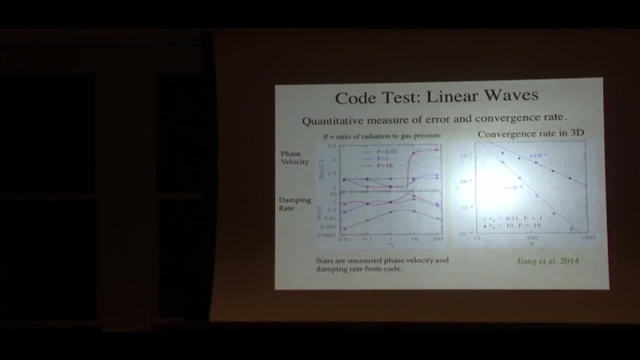 You can semi-analytically solve the equations, compute the dispersion relation for linear waves in a radiation-dominated plasma. You can calculate the phase velocity and damping rate of those waves. And these are the solid lines. in these graphs There's a function of optical depth per wavelength. 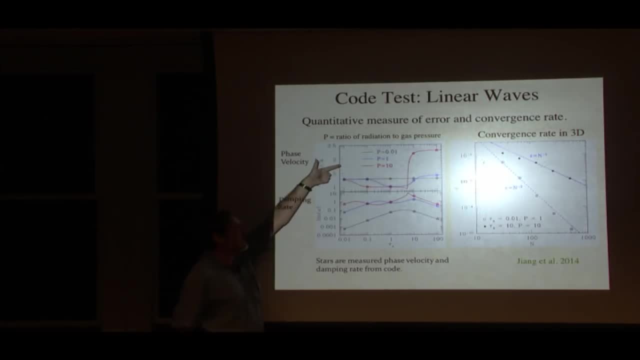 These are the dispersion relations as also a function of the ratio of the gas pressure to the radiation pressure. So over three orders of magnitude in that ratio of radiation to gas pressure we have this dispersion relation And then we can simply do sort of do initial value problems. 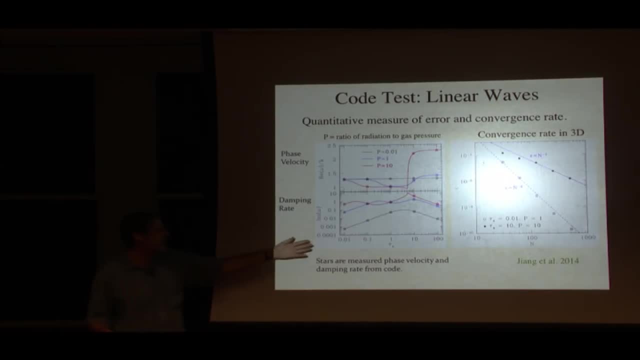 where we just set up a linear wave in a periodic box of some particular wavelength and some particular gas to radiation pressure ratio And then we run it for, say, 10 wave periods And we calculate and measure the phase and damping rate coming from the code, plot it on the curve. 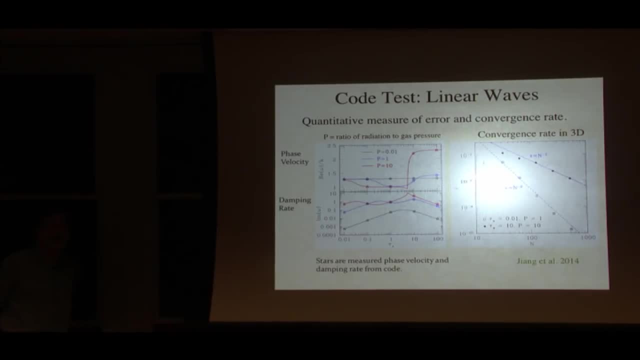 and those are the stars, And they agree extremely well with the linear dispersion relation. But we can do better than that because we have the analytic solution. We can calculate the L1 error between our numerical solution at every grid point and the analytic solution. 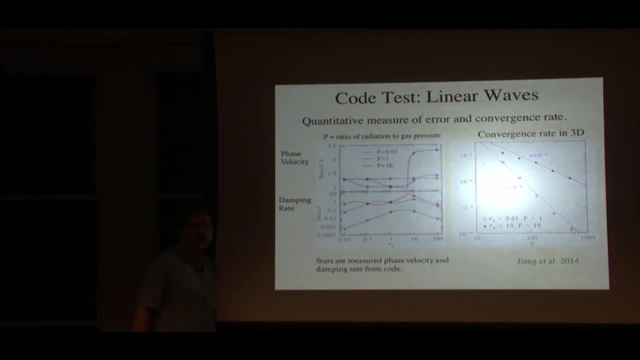 and then change the resolution and make sure the error's converging So we can prove that our method's consistent. it converges to the right answer. we can measure the convergence rate and we have a quantitative measure of the error. So this is one you know good way. 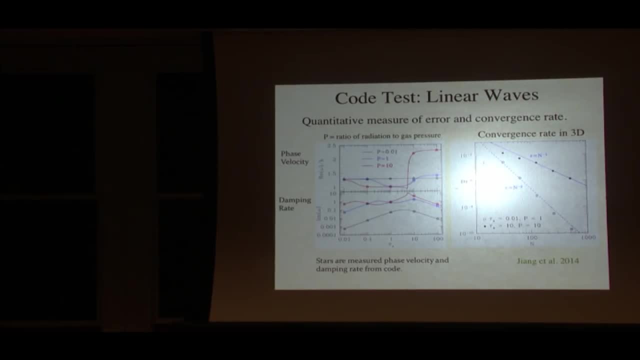 to validate your method and know that it's really working. Yes, Yes, so there's. you can see a big spike in the damping rate. So basically, there's strong radiation damping at particular optical depths and particular gas to radiation pressure ratios, and that's generating that. 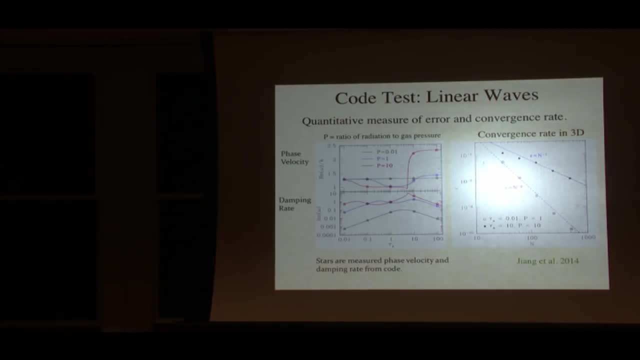 And, of course, you can play the game as much as you like and try to fill in the curve with as many points as you want. At some point, either you or your student gets bored of that, and so this is what we have. These are linear problems, however. 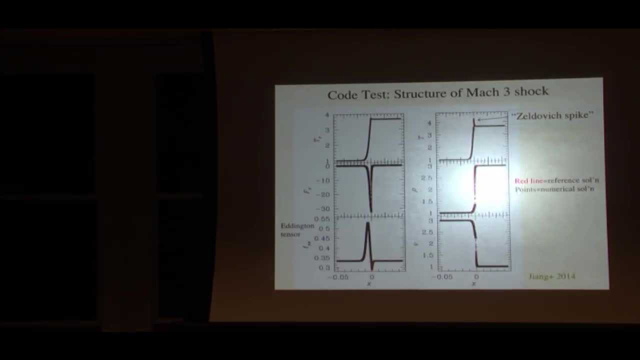 and you worry that? well, maybe in the nonlinear regime the code's gonna break. The only nonlinear solution we found is from Lowry and Morel, who calculated again the semi-analytic solution to the structure of radiation-dominated shocks. 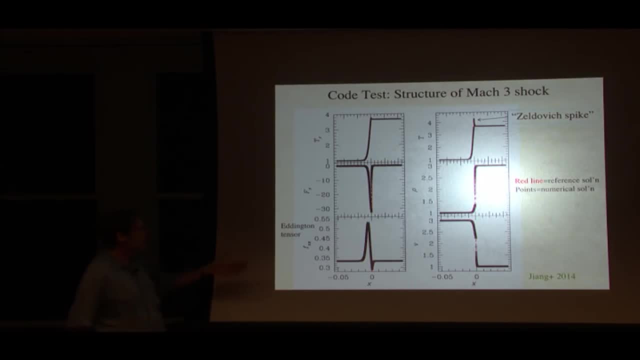 And they gave us those solutions in file format and those are the red dashed lines. So that plots the profiles of, for example, the temperature, the flux, the Eddington tensor, the density and so on, radiation temperature and gas temperature. 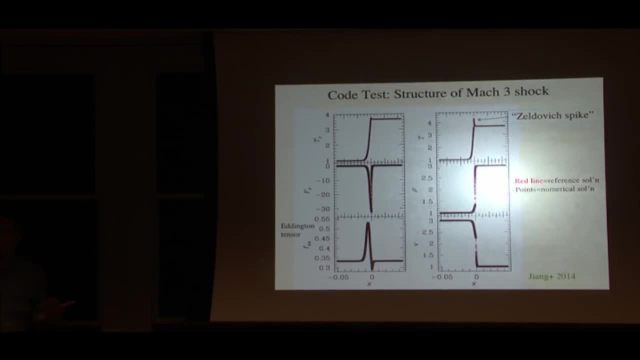 for a shock wave in which radiation is free, streaming upstream of the shock wave and preheating the gas and also cooling downstream and generating the so-called Zeldovich spike. And so again we can compare our numerical solution: set up the shock. 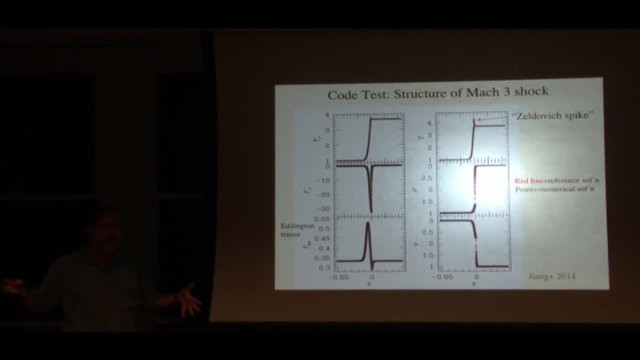 in a domain, in a moving domain, in the frame of the shock, have flow coming in one side, going out the other side, evolve it for many, many, many flow crossing times until it sits a steady state. and then compare the steady state profiles. 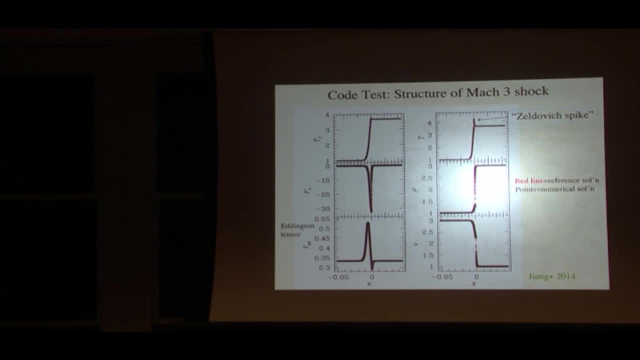 to the analytic solutions And they agree extremely well, which again gives us some confidence. And I would note that things like the Eddington tensor- this is the XX component of the Eddington tensor- does weird things like drop below one-third. 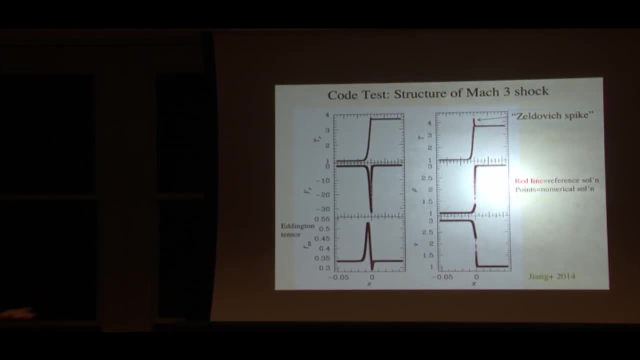 right at the shock front And there's basic physics as to why that happens and why that is. In a plane, parallel shock, you know, angles that are just sort of oblique to the shock wave have more radiation intensity and so are brighter. 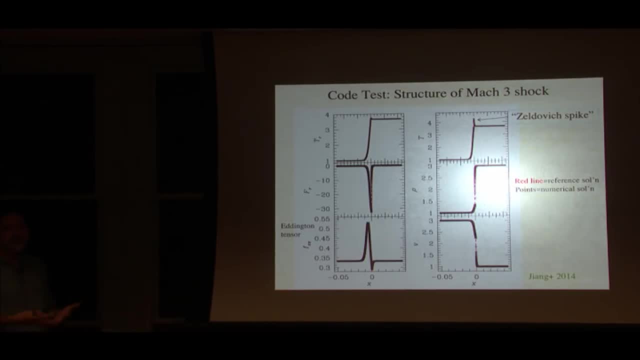 and that leads to a drop of the Eddington tensor there. But any method, any assumption, flux-limited fusion or other closures that assume the Eddington tensor has a certain value- is never going to get this profile correct because it's never going to allow. 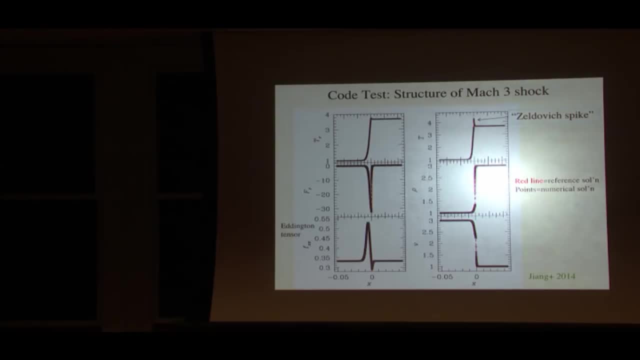 the Eddington tensor to drop below a third. The normal assumption is it's bounded between a third and one, And that's clearly not true. In some radiation flows it's not, It's only one third, And if you don't calculate geometry directly, 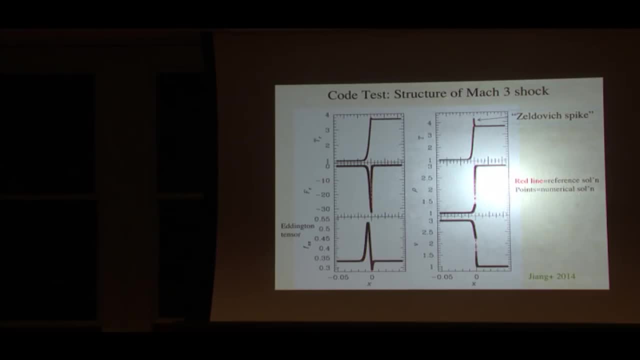 you won't be able to capture that physics. These are non-relativistic shocks. So these are, you know, this Mach number, I think, is like, well, Mach 3.. There you go, Yeah, But it's still a radiation-dominated flow. 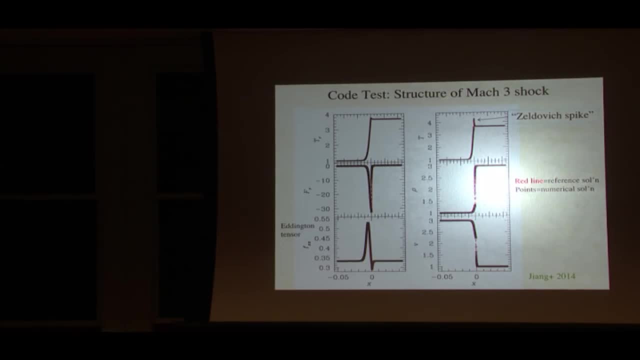 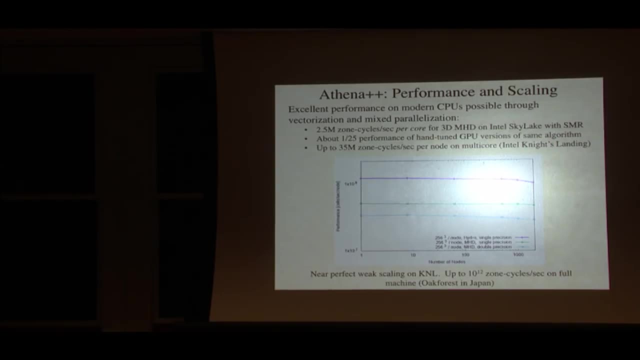 but non-relativistic, And the other aspect of these solutions is good scaling and good efficiency. So another aspect of Athena++ is we spent a lot of time writing code that would easily vectorize and take advantage of modern processor design, And so, after a lot of work, 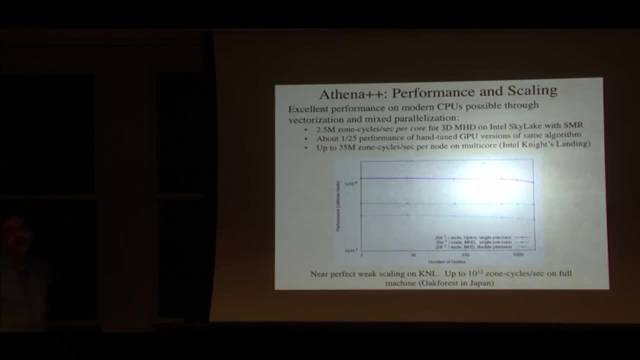 we get about 1- 25th the performance of a GPU per core on a standard Intel CPU, And since CPUs nowadays come with 14,, 16, 28 cores, then one CPU is performing similarly to one GPU for this kind of algorithm. 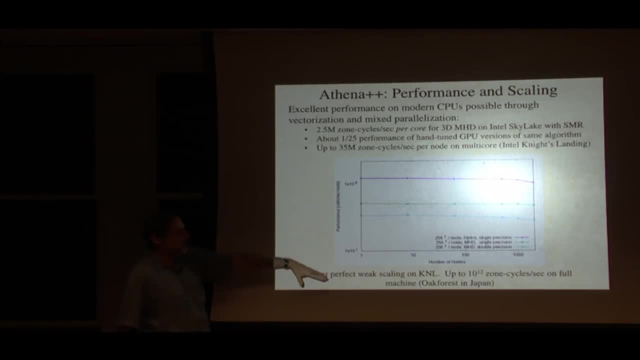 And, moreover, the scaling remains the same. It remains extremely good. So this is a Intel Knights Landing machine which has up to 8,000 nodes. This is the performance per node compared to the single-node performance. Perfect, weak scaling is a flat line. 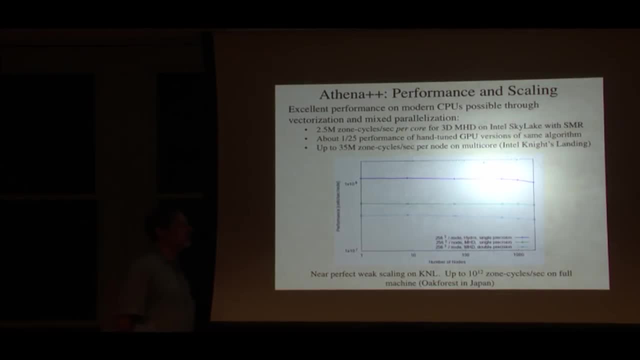 and it remains extremely flat. In fact, this is actually a networking error that Kengo found on the full machine, and so that point is a little bit better in the more recent plots. But the point is, these processors, are these multi-core processors? 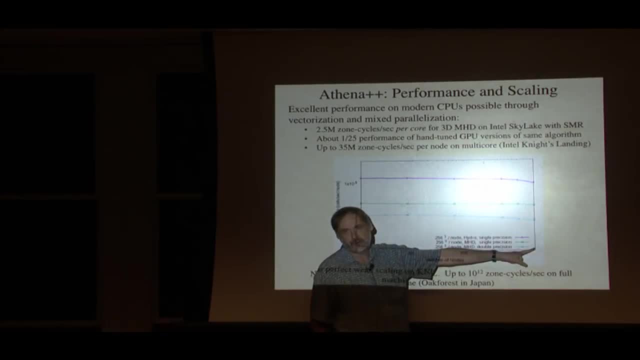 They have like 64 cores. this is half a million cores out here. We're getting better than 98% efficiency, So we can use a very large machine and that's good, because these are expensive calculations and you need to be able to exploit modern architecture. 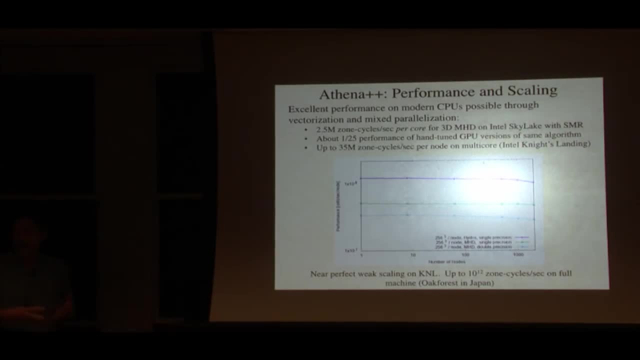 You know, what GPUs are great for- and there's many experts here on GPUs- is that there's some very, very large GPU machines nowadays that are probably underutilized. So those with GPU codes- Evan and others- are in great positions to really exploit. 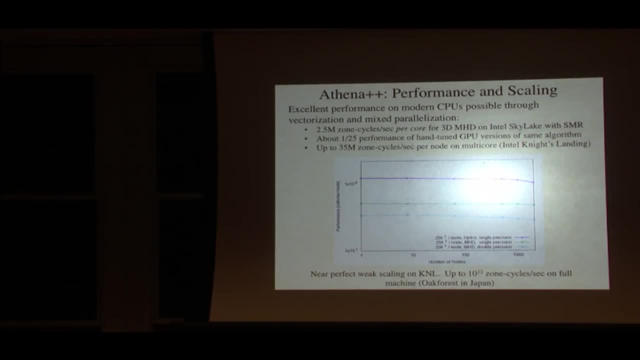 the available time on GPUs and GPU machines coming forward, But there is an exascale machine coming out in 2021, which is going to be built on Intel processors and we hope we're well-placed to take advantage of that architecture in the future. 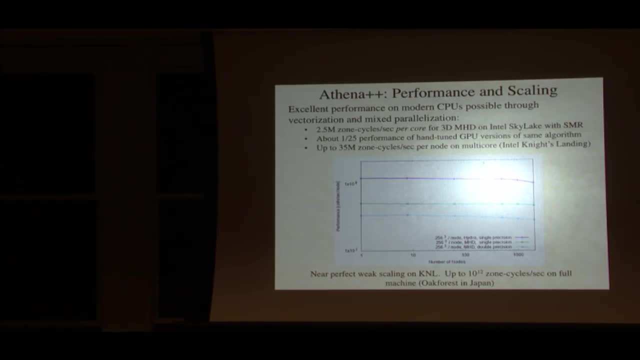 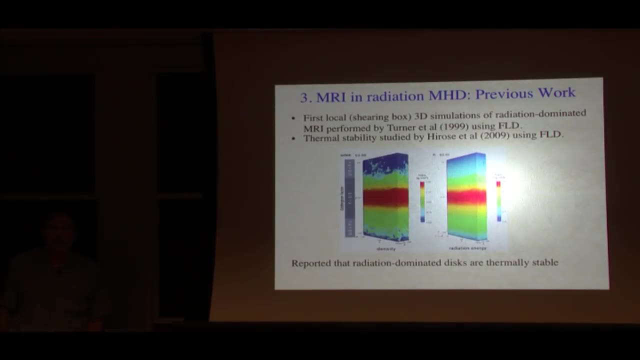 So we have the numerical algorithms developed, and so let's turn to some results. But first let me say a few things about what's been done previously. I mean, we're not the only ones working on this problem, and indeed for quite some time. 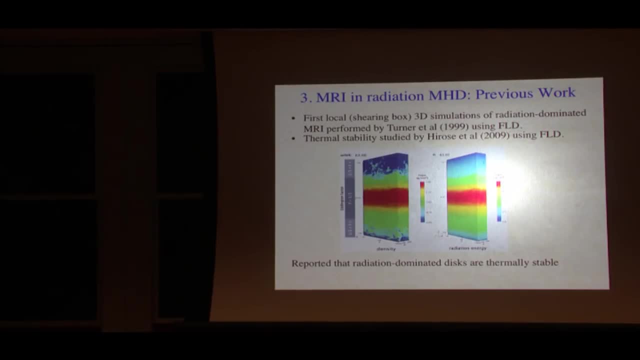 people have been interested in this problem, Going back embarrassingly, 20 years, where the first calculations of the saturation of the MRI was studied in a local shearing box by Neil Turner, using the Zeus code, in fact, And then 10 years later. 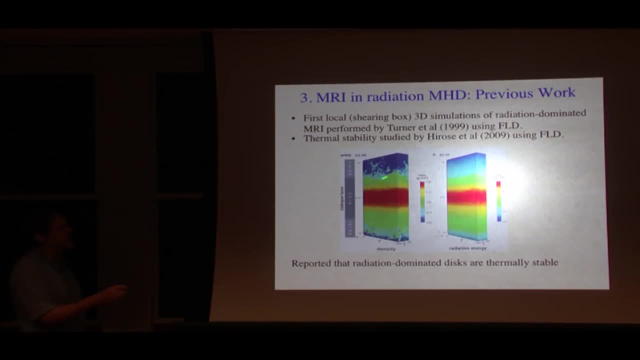 Hirose et al and collaborators used that same code to study the thermal stability of the accretion disks using local shearing boxes, so-called stratified shearing boxes, where the density varies with vertical position. So you have MRI turbulence generating heat and dissipation in the mid-plane. 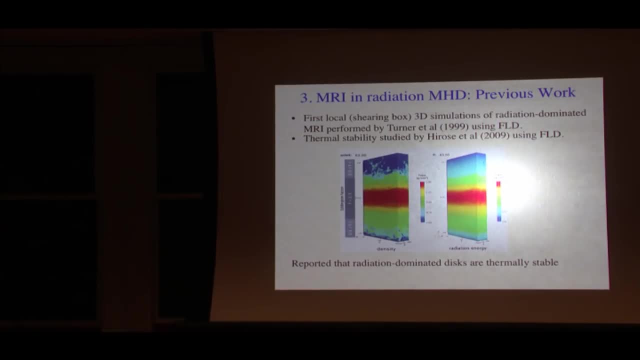 and you follow the radiation transport, the cooling of the disk and you're looking for thermal stability Because you know, motivated by the famous papers that predict the disks to be thermally unstable, alpha disks to be thermally unstable in the radiation-dominated regime, 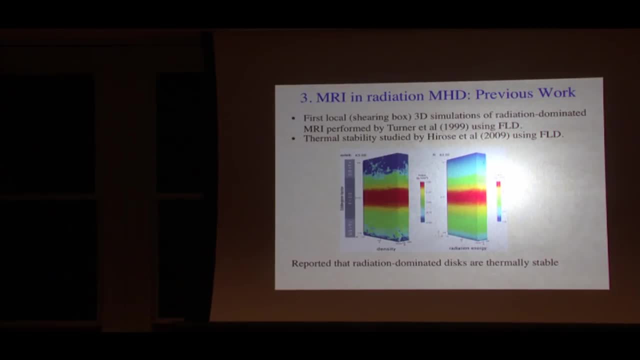 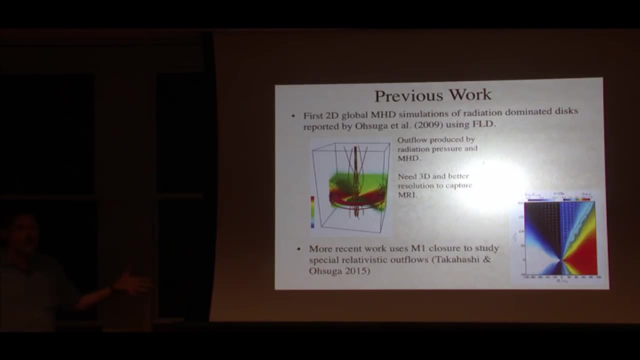 they reported these disks were actually thermally stable when they had MRI turbulence producing a dissipation. So this was some of the most important first work. The first global calculations that went beyond the shearing box, I think were by Ken Asuga and collaborators. 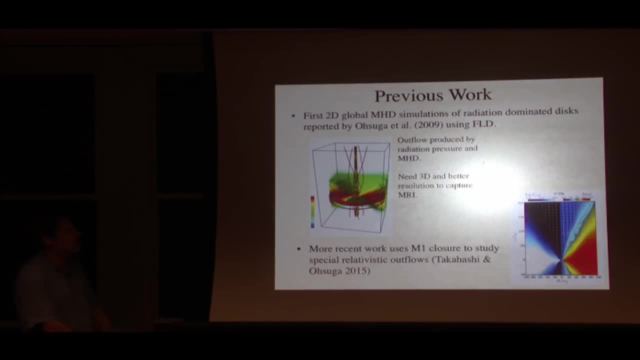 who did 2D calculations showing the production of outflows by radiation pressure and MHD. These really needed to be extended to 3D to follow the turbulence generated by the MRI, with better resolution to capture the turbulence, And they've been working a lot on this problem today. 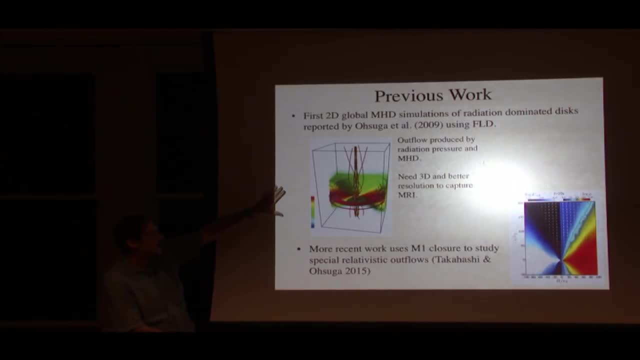 Nowadays they're adopting the M1 closure instead of flux-limited diffusion. They've been doing special relativistic flows. They have a lot of papers Recently. they're a very active group looking at accretion onto black holes and neutron stars. 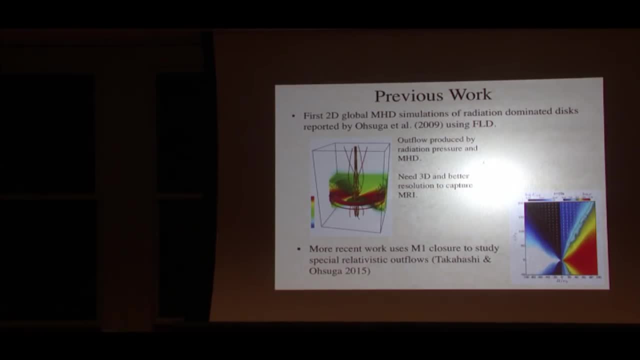 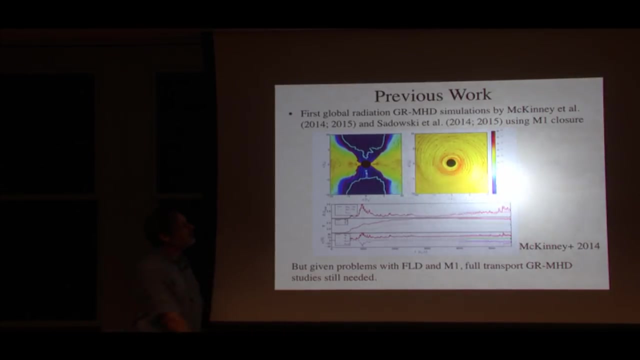 And so there's a very productive group associated with Ken and his collaborators producing these results, And I would say they were the first to do these in fully global calculations. The first global general relativistic calculations, I think, were by John McKinney and Oleg Sadowski. 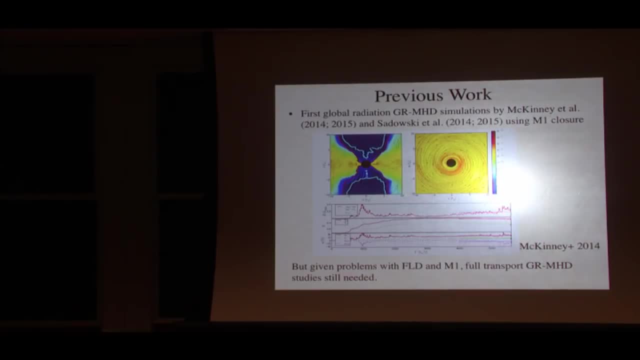 roughly at the same time using two different codes, back in 2014-15.. They have done full GR MHD calculations With the radiation transport approximated using this M1 closure: a two-moment closure with this ad hoc M1 closure. 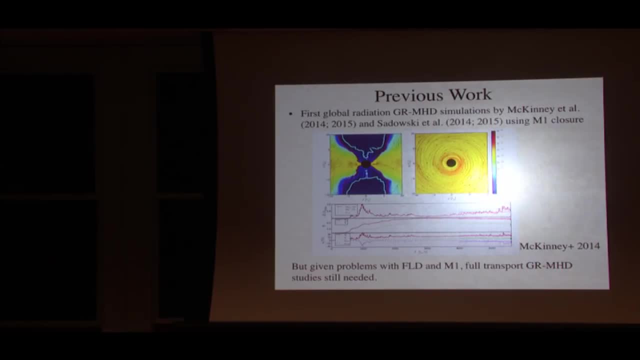 for the radiation field. Now that enabled them to do GR, because you could extend M1 to fully GR transport fairly straightforwardly, And so they're the first to be able to do the GR, And so here's a snapshot, for example: 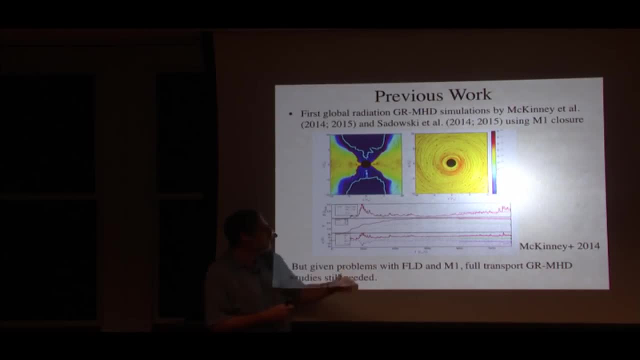 of the density field in the poloidal and equatorial plane. And then you probably can't see the bottom here, but they plot accretion rates and efficiencies versus time And I'm sure you really can't see this, but I can't see it. 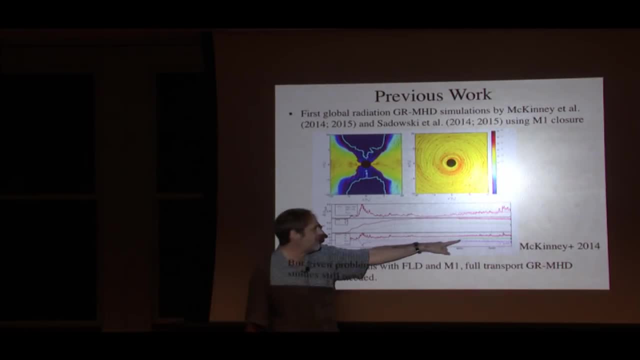 Eta, the blue, this light cyan line. here is the radiation efficiency, the fraction of the energy radiated away compared to the energy released by accretion, And that's zero, And so they get a very, very small efficiency. 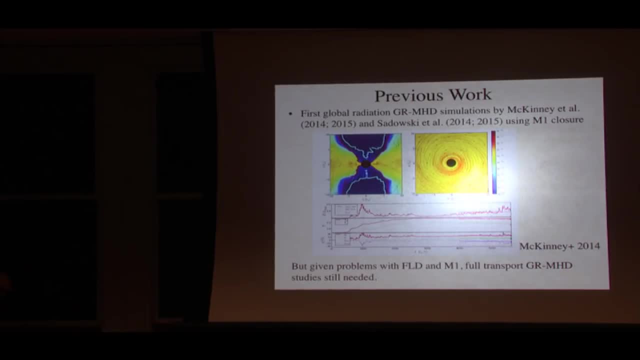 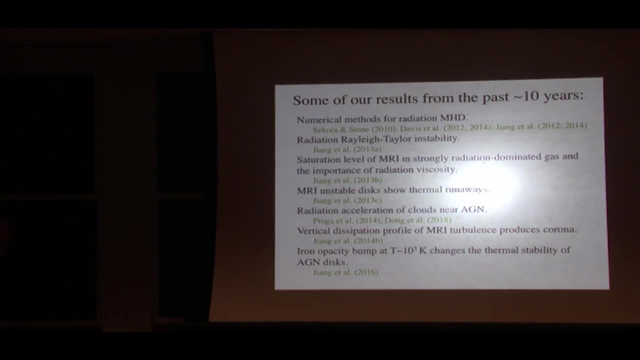 less than 1% for these super-Eddington accretion flows using these M1 methods, And so we'll return to that. So we've also been working on this, And by we I mean most of the work, hard lifting, being done by collaborators. 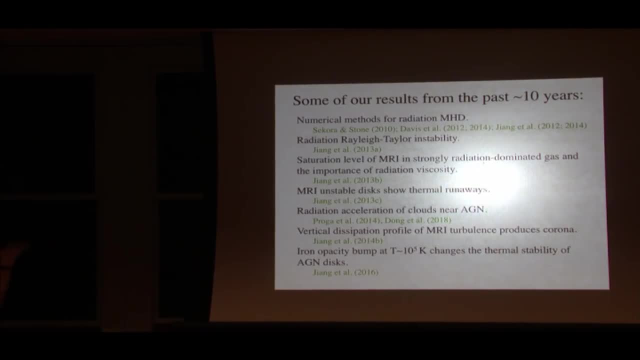 And so useful, for me at least, to sort of catalog some of these results that I've presented before and I won't present here. So of course the first step was developing the numerical methods and publishing those First problem that Yanfei did. 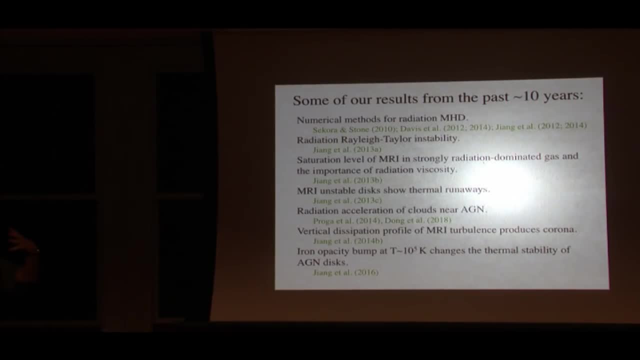 was looking at the radiation Rayleigh-Taylor instability, where you have a fluid supported by radiation against gravity. He then looked at the saturation of the MRI and strongly radiation-dominated gas where the radiation pressure was, say, 10 to the 4,, 10 to the 5 times the gas pressure. 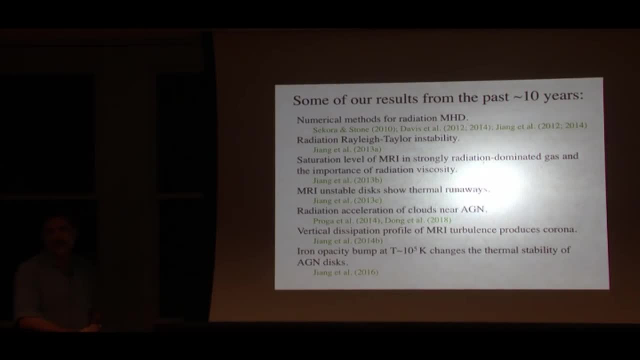 and discovered that radiation viscosity plays a big role in damping the MRI in that situation. He had repeated the stratified disc calculations and showed that discs in fact do show thermal runaway, in contradiction to the previous results by Hirose et al. And it turned out the difference was partially due. 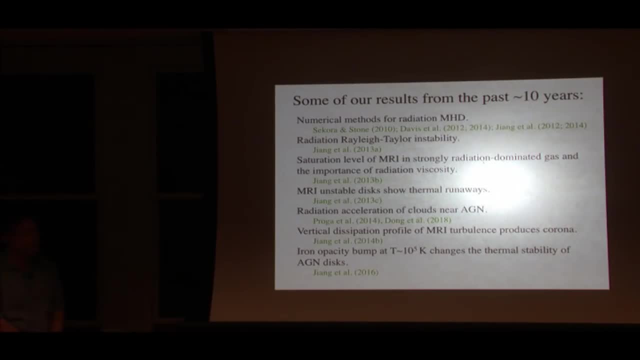 to the numerical algorithms we're using these more advanced radiation transport algorithms, but also the properties of the shearing box they were using were different than what we're using and that resulted in this difference. Daniel Progan, collaborator, has been using this code. 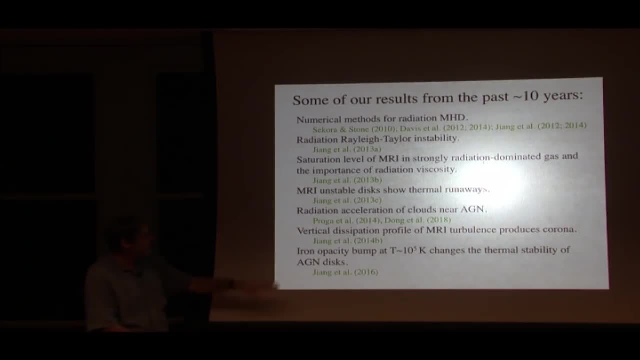 to look at acceleration of clouds around AGN. We've also written a paper about how you can form corona in shearing box calculations due to the dissipation of energy above the photosphere. I'll return to that again later in these global simulations. 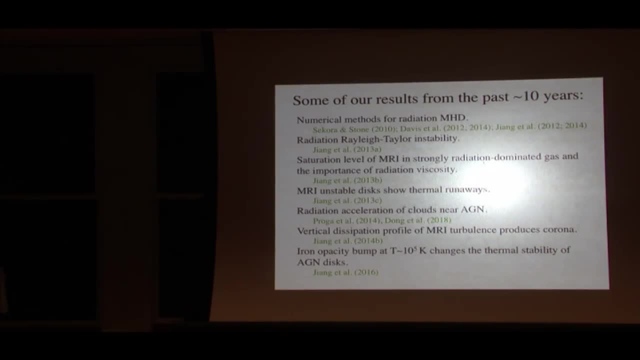 And then most recently, as part of a project to study convection in stars, in very, very hot stars, Yanfei's implemented a more realistic opacity table. this gets back to Michael's question that actually around temperatures of 10 to the 5 Kelvin. not all of the iron is completely ionized. There are some trace amounts of highly ionized species of iron left around, And iron has millions and millions and millions of lines, and the combination of all those spectral lines, transitions, adds to the overall opacity by a factor of two or three. 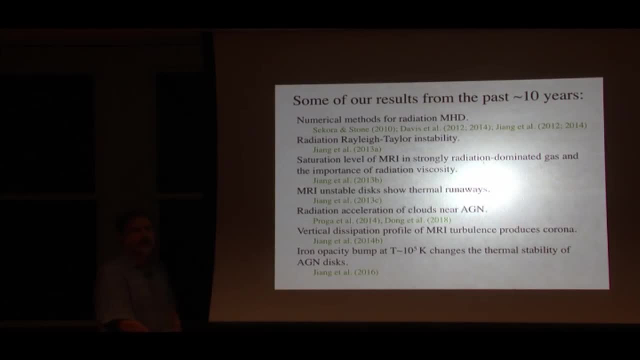 The so-called iron opacity bump that kicks in around 10 to the 5 Kelvin And it turns out that that changes the thermal stability. When you include this iron opacity bump, you can change the thermal stability properties of the disk. It only really applies to AGN disks. 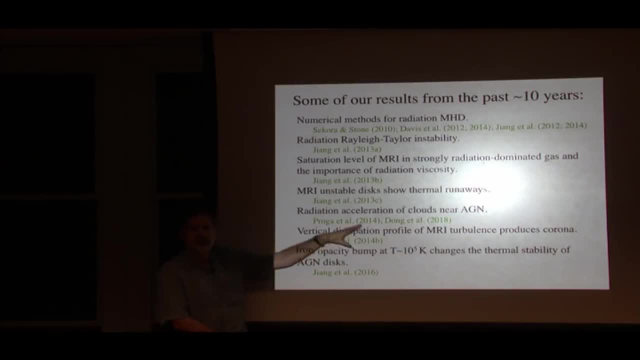 because they're the only ones that sort of sit in this temperature range. X-ray binaries: the temperature is much, much higher and it's fully ionized and this effect doesn't occur there. But it's another indication that there's a lot of physics to be included here. 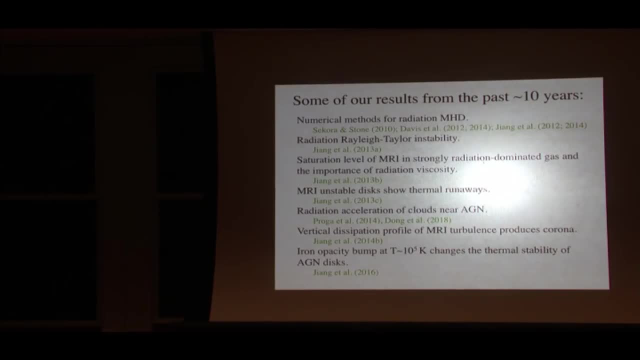 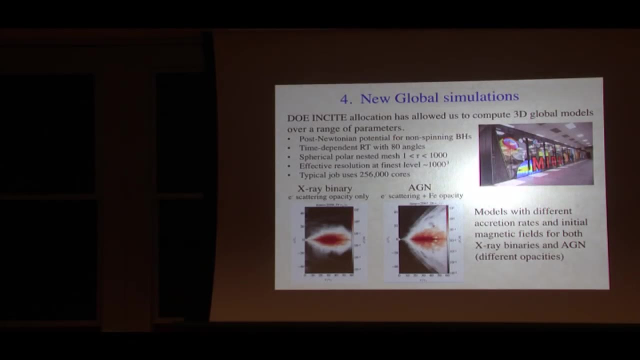 and that opacity is going to make a difference. So that's all the stuff that I've talked about before and I'm not going to talk about now. I'm going to talk about these global calculations that we've done over the last couple of years. 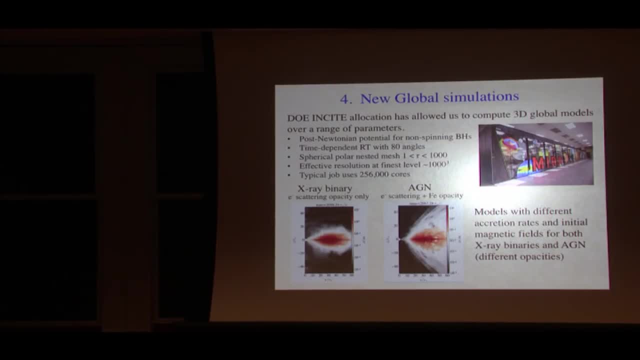 both for super-Eddington and, more recently, sub-Eddington flows. They were enabled by a large allocation from the DOE Insight Program. It gave us 100 million core hours on one of the largest machines in the country called MIRA Computer centers normally charge. 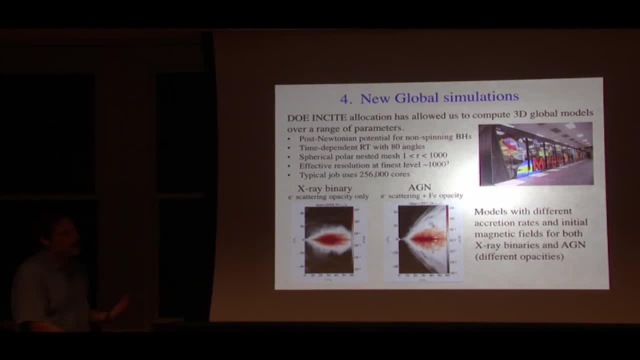 computer time at 5 cents a core hour. So 100 million core hours. that was a $5 million research grant for one year on this machine. That's great. And also it means students and post-docs who run your code for two weeks on Perseus. 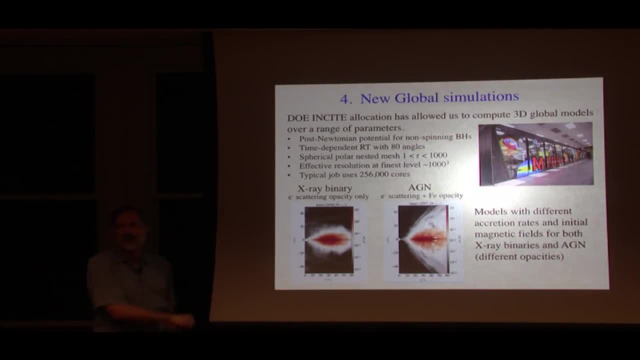 and then realize, oh, darn it, I used the wrong parameter. Kill the job. let's start again. 5 cents a core hour, Remember, computing does really cost, So we would never be able to do this using local resources. It really requires these national centers to do it. 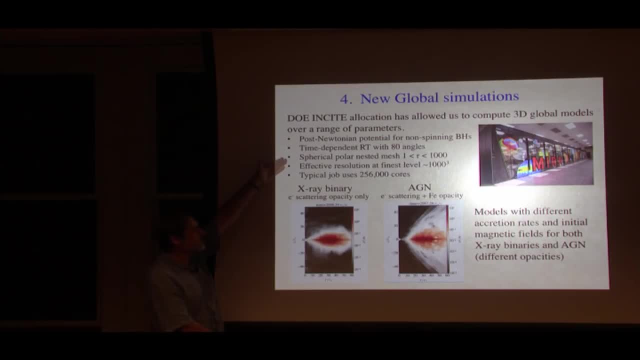 This allowed us to look at spherical polar meshes with three orders of magnitude and radius, So we have a very large dynamic range in the radial direction. We have 80 angles at every single grid point, So we have good resolution of the radiation field with angle. 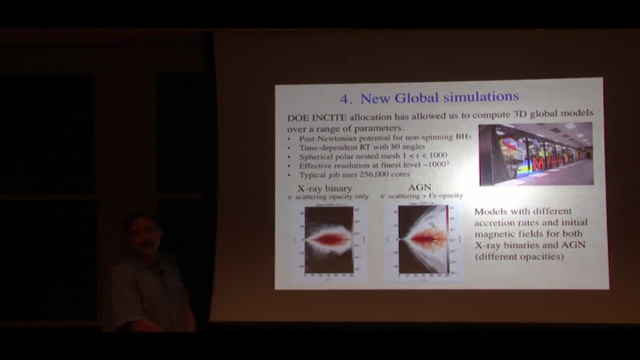 We're using these nested meshes to reach effective resolutions of 1,000 cubed. at least 16 points per scale height in the disk, even for the sub-Eddington disks, which is enough to resolve the MRI wavelengths. Typical jobs use about a quarter million cores. 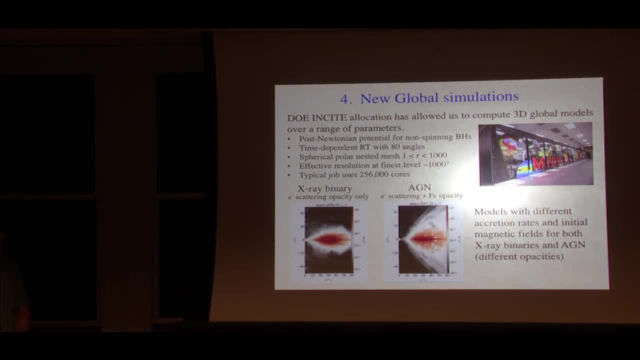 And it was enough time to be able to do a full parameter survey where we vary magnetic field geometry, the surface density, to give us different mass accretion rates. We've also considered X-ray binaries which only have electron scattering opacity, and the AGN, where we both include electron scattering. 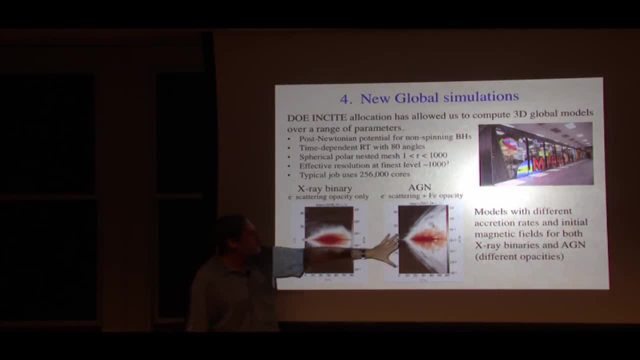 and this iron opacity bump. I'm only going to focus on the AGN results today, but I will talk about what results with different surface densities and fields that give you different mass accretion rates. Yes, These are all continuum opacity only. 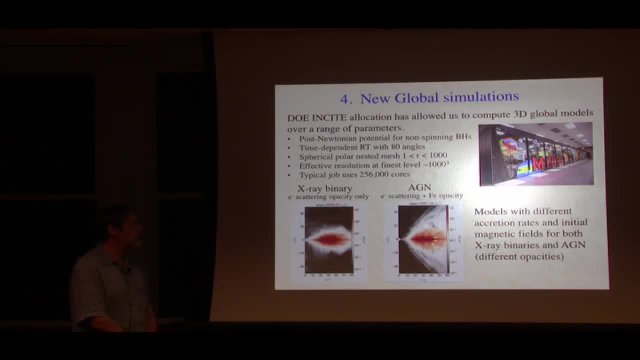 so just gray, Just gray, Which you know, until you get farther out, is still pretty good, because it's mostly electron scattering or, in this, iron opacity bump, you can still treat it with gray. But for the future, for the future getting farther out in the disk, 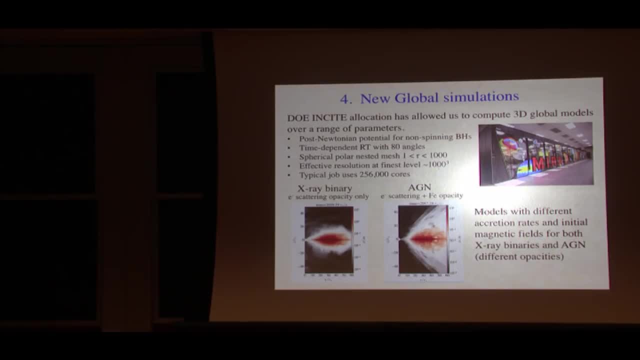 where you have to worry about lines and other things, is very, very important. Sorry, which symmetry? It's actually not exactly symmetric, and so there is turbulence and there's a global sort of symmetry, but it's not. you know, overall the density. 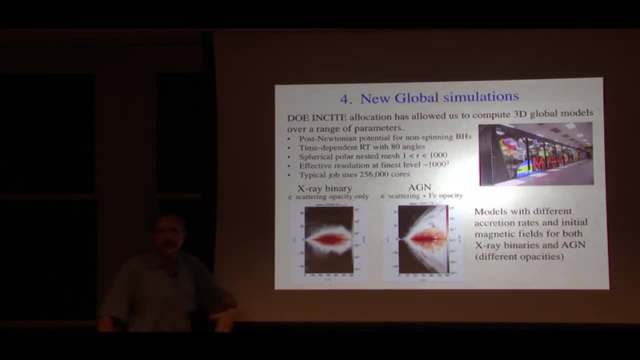 But if you zoom in you know there's motion across it. It's the full four pi steradians in the spherical polar mesh. There's no quadrants or symmetries assumed during the full problem. Okay, so what do these flows look like? 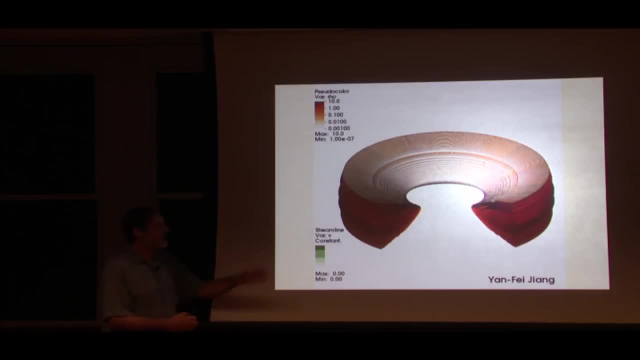 We start with this bound rotationally supported torus of plasma with a weak magnetic field. These are surface densities of, or surface isosurfaces of the density. We run the calculation. It goes MRN stable in the inner regions first. 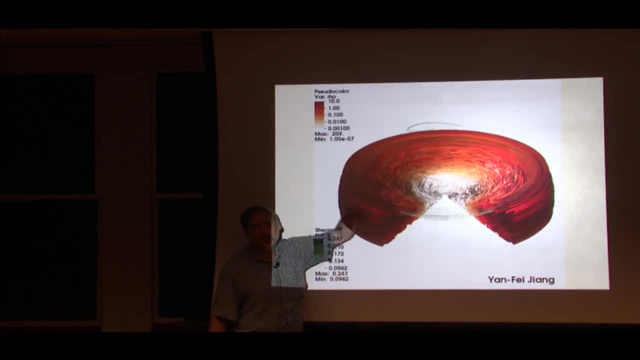 because the time scales there are the shortest, Generates accretion inwards from angular momentum transport from the turbulence And then eventually the entire flow, including the outflow from the outer regions, becomes turbulent and it settles down into a quasi-steady accretion flow. 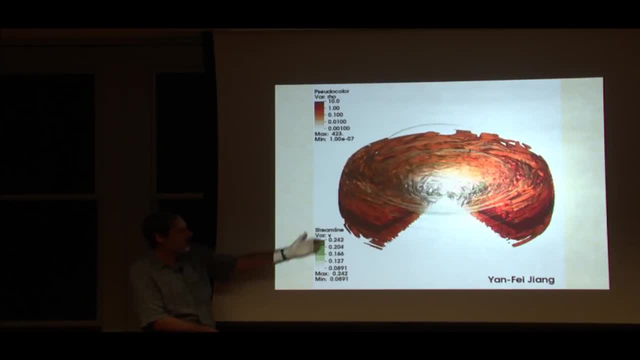 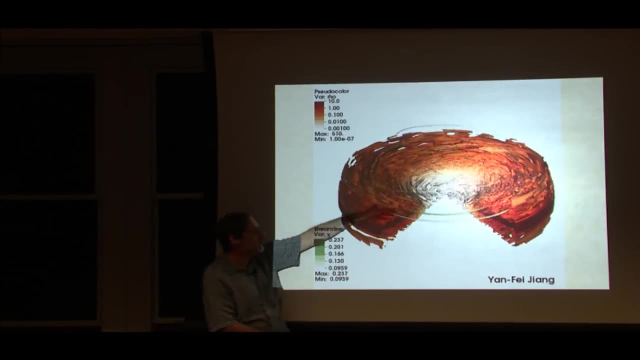 Typically we run these for ten or more orbits in the outer edge of the disk, So that's long enough for the MRI to saturate everywhere and to generate an accretion flow where matter is being self-consistently fed in by the angular momentum transport. 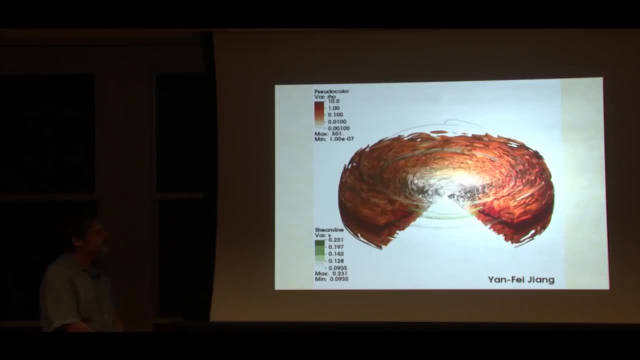 associated with the MRI turbulence in the bulk of the flow. The streamlines are the lines there and you do see some outflow here, but they're both. you know, surprise, surprise, They're mostly azimuthal because of the rotation of the flow. 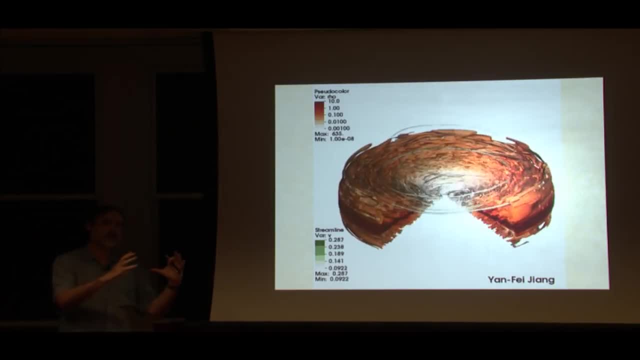 That was just the you know. so it's just a self-contained torus of material. The boundary of the mesh is, in fact, another order of magnitude farther away, because we, you know, material will move to larger radii, as it. you know, as matter falls in. 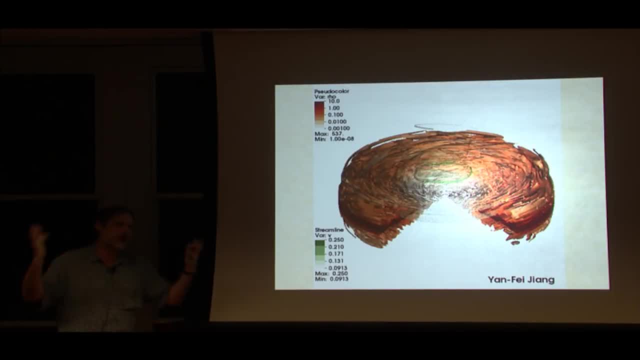 some has to go out. Moreover, you generate winds and outflows from the radiation magnetic field. We want to be able to capture that. So the outer boundary is much, much farther away. This particular case, the magnetic field, I think, was simply parallel. 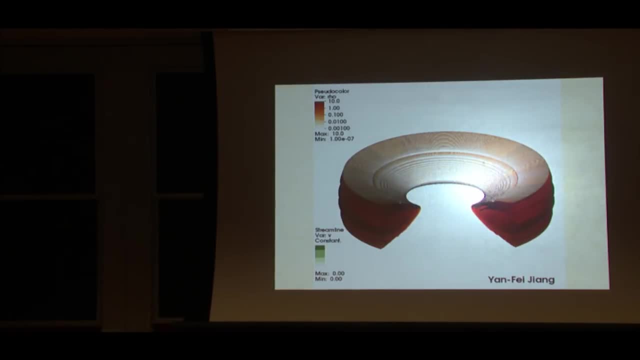 to the isosurfaces of the density. So there's field loops inside it and no net flux over the volume of the terrain And it sort of settles down into this rotationally turbulent flow. Maybe for today, when Florence is coming by, this is, you know, our nice hurricane. 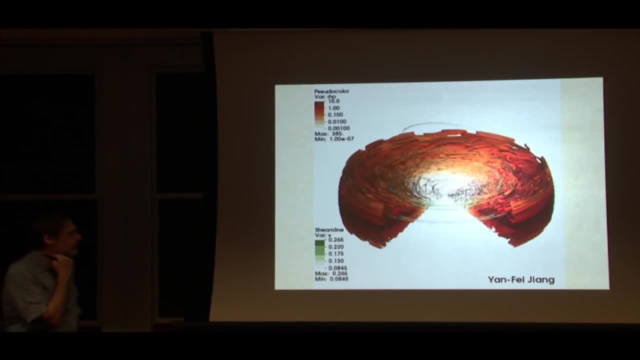 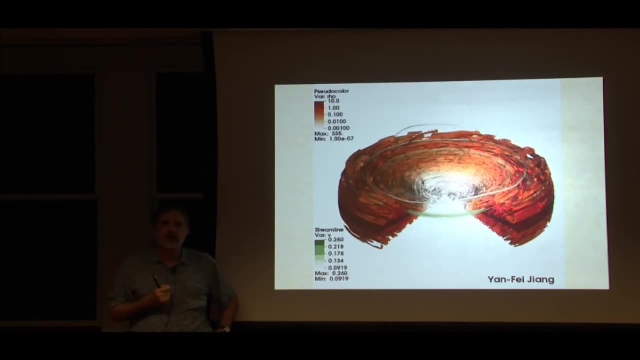 Yes, It's stationary. So we're using this post-Newtonian approximation. We're not doing full GR in the middle, meaning we can't treat spinning black holes at the middle. We do have an interstable circular orbit, just like a Horschel potential. 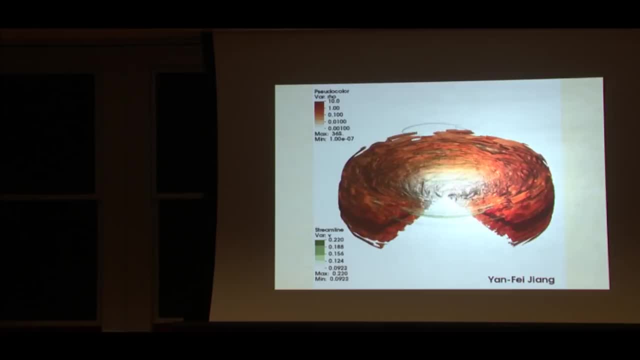 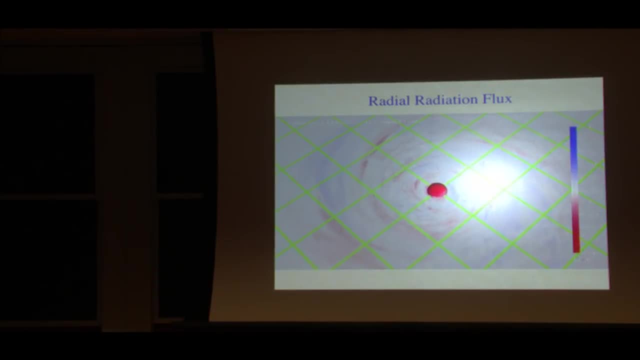 but we don't have the ability in this approach to do spinning black holes. Okay, so visualizing these flows is complicated. Here's another animation to try to help you see what's going on. This shows you the radiation flux, the radial component of the radiation flux. 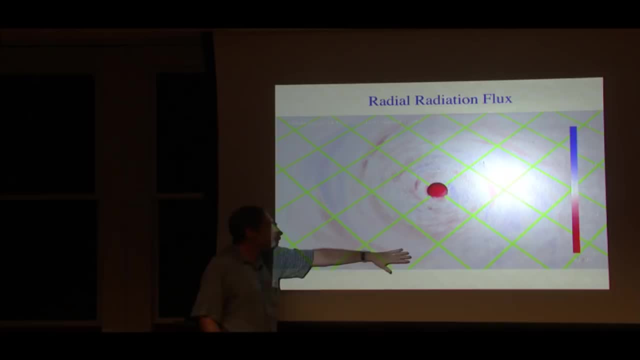 Blue is outward, Red is inward. It's going to show you the radiation flux on an equatorial slice and on a sphere which is going to grow. It's going to sort of slice through the volume in time. It's going to move farther out. 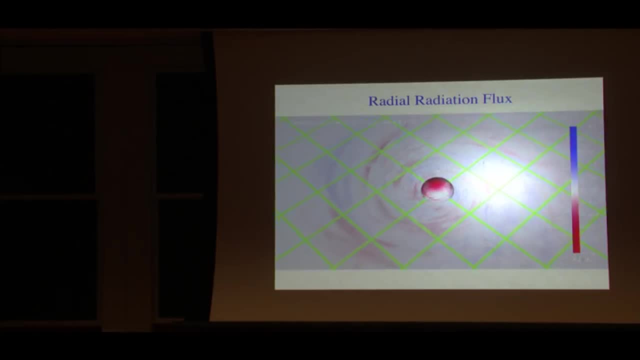 And then we're going to open up this sphere and see what's going on inside. Let's play it away So you can see that there's outward radiation flux. you know, in the upper polar regions- The midplane is turbulent- There's both inward and outward flux. 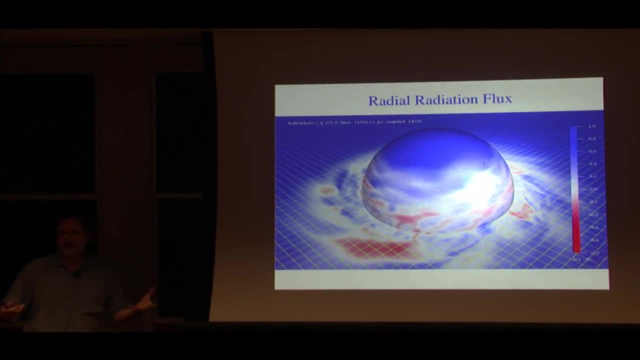 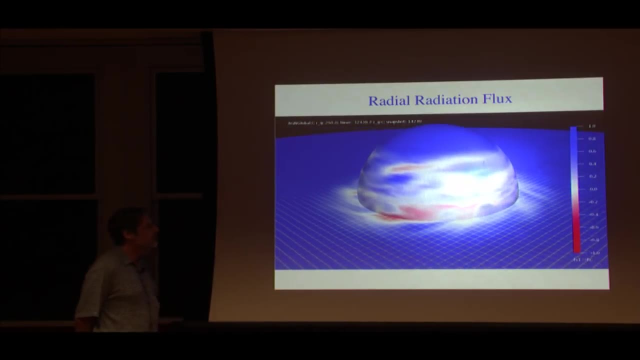 The inward flux is associated with radiation in optically thick regions which is trapped and moving inwards with the flow, and that gives you inward radiation flux. We get to the outer part of the disk at 300 RG and we're going to open it up. 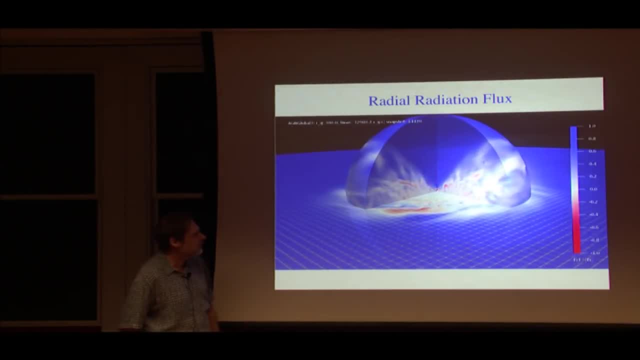 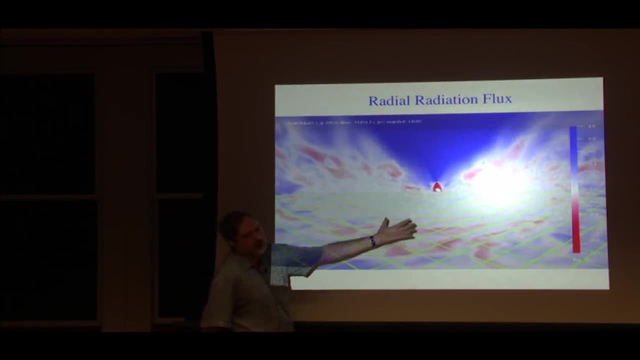 and the disk is continuing to evolve. So you can see the turbulence and now you can see in a poloidal slice the distribution of the radiation field, the orbital motion of the disk at the equatorial plane, and so on. This is an animation made. 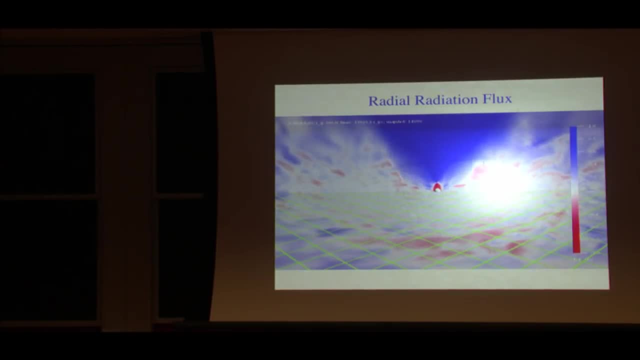 at the NASA Supercomputer Center from some of the data that Yanfei had generated from some of his calculations. So generically turbulence in the midplane of the disk and strong radiation outflows above the photosphere for this particular calculation. So we can generate super Eddington accretion generically. We can't specify what the mass accretion rate is. It's generated self-consistently, but by using a large enough surface area, mass density and a strong enough magnetic field, you get super Eddington accretion rate. 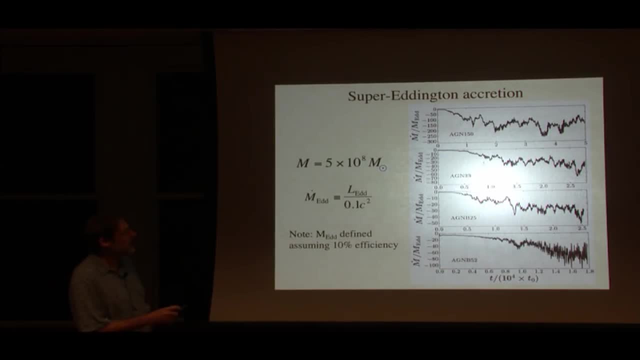 This is the mass accretion rate versus time for four different models. The number at the end is the time average mass accretion rate for the last few hundred or few thousand, I should say, light crossing times in the model, So measured in terms of the Eddington mass accretion rate. which itself is defined using a 10% efficiency. So you don't quite know what the radiation efficiency is. People generically assume 10%. With that assumption you can calculate m, dot, Eddington, and this is the mass accretion rate we observe. 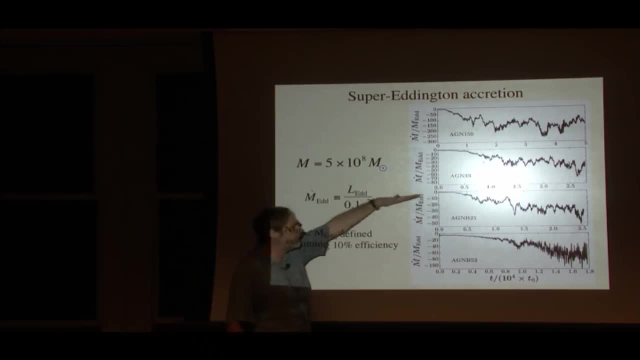 normalized by that value. So generically the mass accretion rate increases and then becomes highly fluctuating but quasi steady state and you can get a wide range of values in the super Eddington regime. So what is the physics? 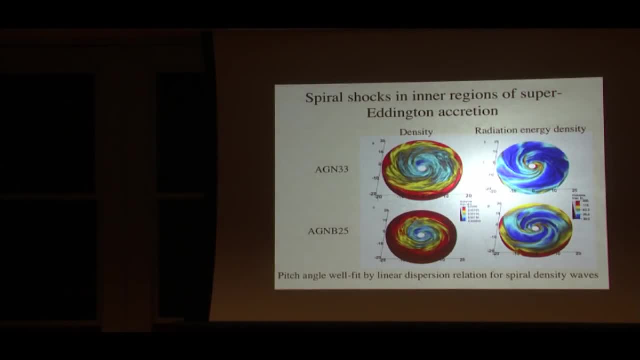 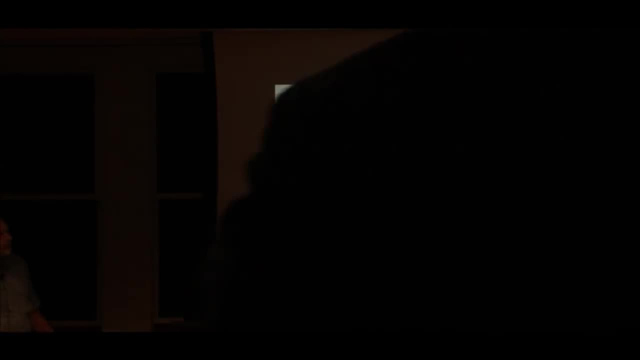 So we get super Eddington accretion for sure. What's the physics of this? One important aspect is the emergence of spiral density waves In the very inner regions of the flow, so the inner 20 RG of the flow, especially in the radiation energy density. 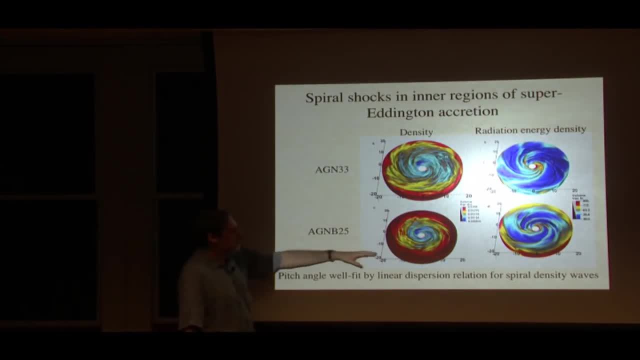 you can see these spiral modes which end up contributing significantly, in fact dominating in some cases, the angular momentum transport in the flow. So these are modes that have been excited by the turbulence, which are exciting spiral waves which then propagate inward, steep into the shocks. 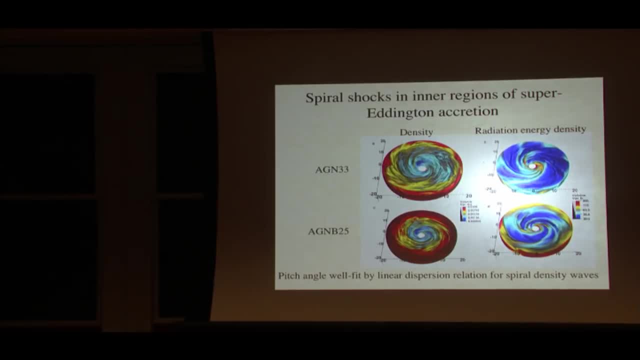 and give you these spiral modes And, to be honest, there's still work to be done in understanding exactly which frequency and which modes are being produced here. This is not seen without outside of these super Eddington flows. this has never been seen before. 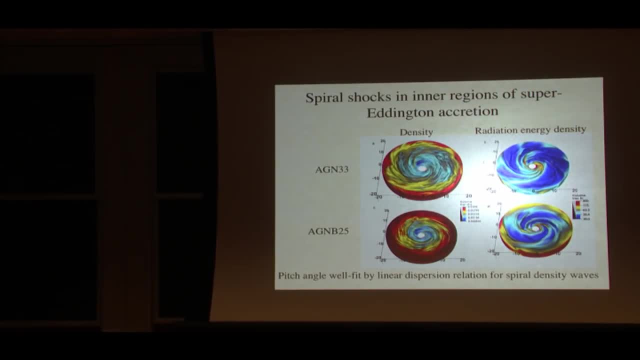 This seems to be a unique property of super Eddington accretion disks, where the radiation energy density dominates so strongly In the mid plane. they're going to mostly follow these flows, So they're mostly being. now there is a fluctuating part of the field B. 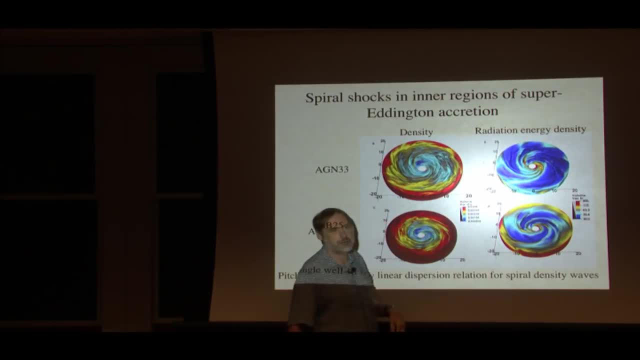 but it's only 10% or so that the toroidal component is being drawn out here. Yes, So these calculations are independent of the mass. We can scale them to any mass we like. So yes, this would be super Eddington for a neutron star. 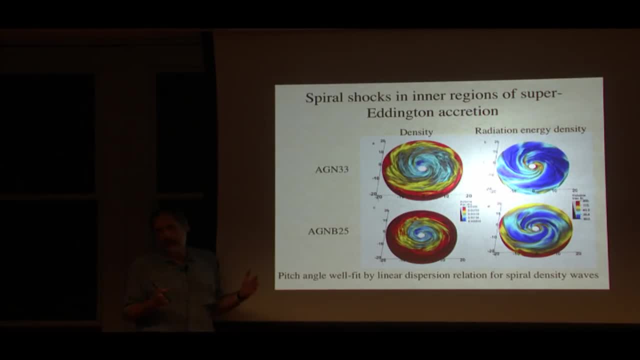 The only worry would be that the opacity sources might be different, because the neutron star temperatures, the flows in a neutron star accretion flow, the temperatures there would be much different than here, And so you might need to not include the iron opacity. 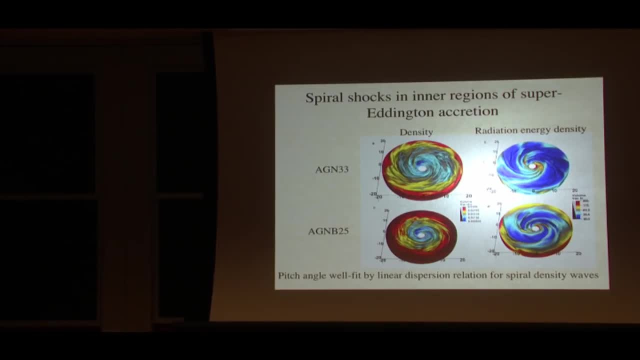 for example, in the neutron star flows. Of course, the biggest difference in neutron stars is the surface And the flow is hitting the surface and the radiation field has to get out from that. And these are black holes in the sense that material goes in the inner boundary. 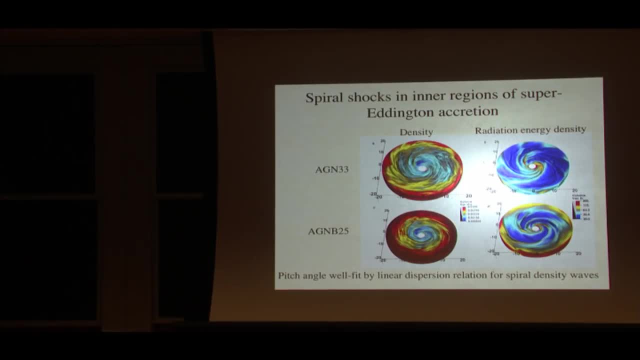 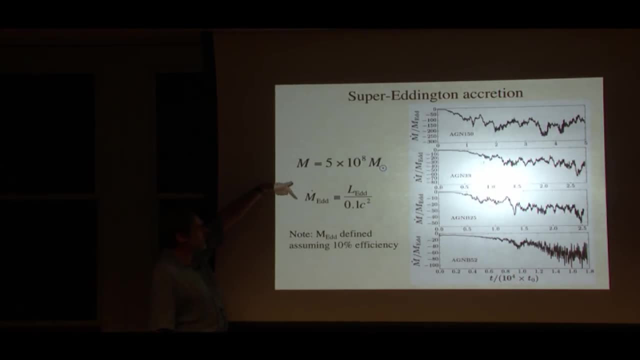 and radiation goes through the inner boundary and it doesn't come back. No, We've scaled this for a five times ten to the eighth solar mass black hole. These would be the mass accretion rates. It stays the same exactly. 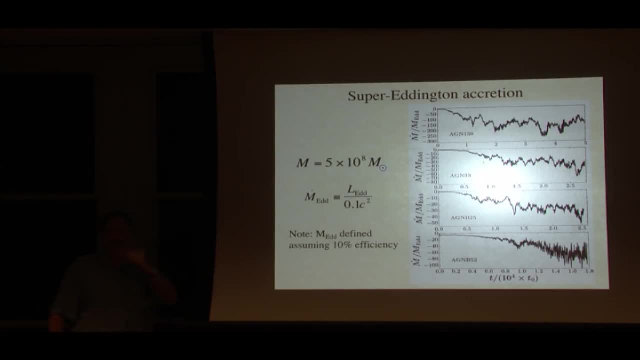 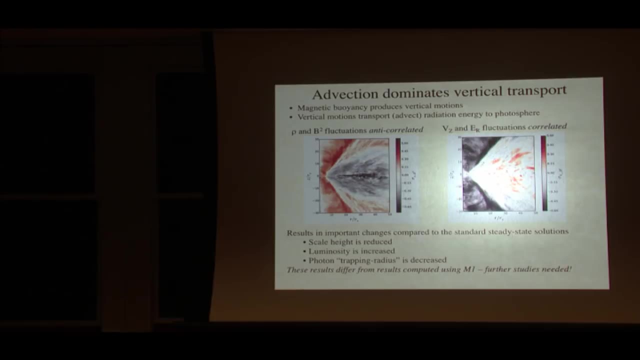 So these numbers are provided for your convenience. So I think one of the most important results to come from this is the role of turbulent transport of radiation energy density. There's an interesting chain of correlations that come up to play here. So the MHD turbulence generates. a strongly varying magnetic field And that generates regions of high magnetic field and weak magnetic field. In regions of high magnetic field the density is lower, so that the total pressure remains roughly constant. So that means there's an anti-correlation between the density and magnetic energy fluctuations. 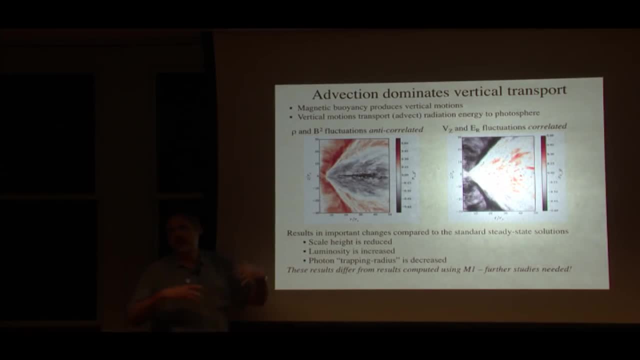 Where the magnetic field is strong, the density is small. There's basically low density bubbles. where there's strong magnetic field, Those bubbles are buoyant and they try to rise out of the disk. that generates a vertical velocity And, moreover, low density bubbles get filled with radiation. 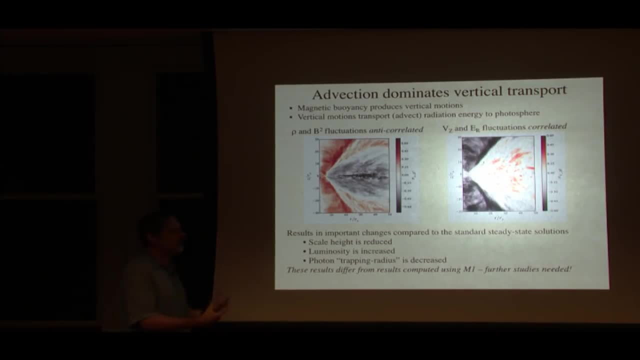 The radiation produces pockets of low density and high radiation energy density And those pockets are preferentially moving outwards towards the photosphere And they simply transport the radiation along with them. So there's a strong positive correlation between the vertical velocity and the radiation energy density fluctuations. 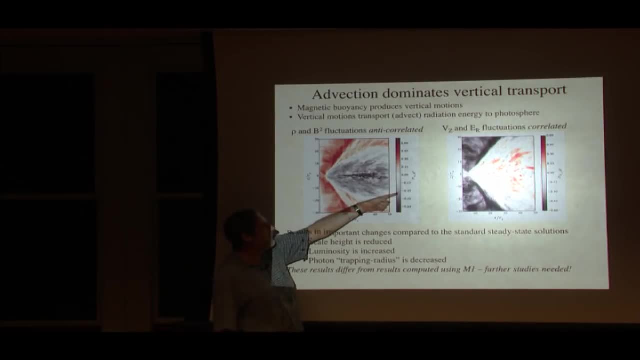 So these two plots show you the correlation functions. Black is a negative correlation, Red is a positive correlation. So you can see these correlations emerging self-consistently, And that means there's a significant amount of cooling due to what amounts to convection. 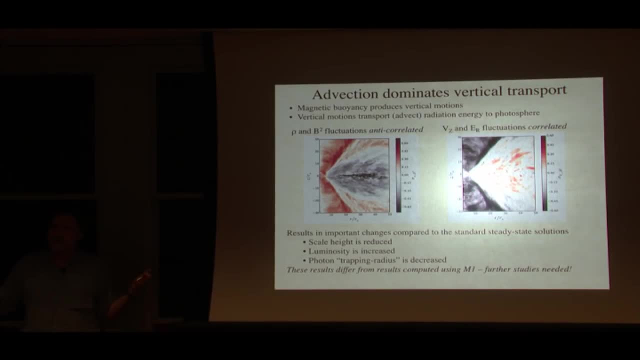 That these correlations between the velocity fluctuations and radiation energy fluctuations are transporting energy outwards and that's producing more cooling. Standard analytic slim disk models assume only radiation diffusion for cooling, And here clearly turbulent transport is contributing significantly. In fact it's dominant over radiation diffusion. 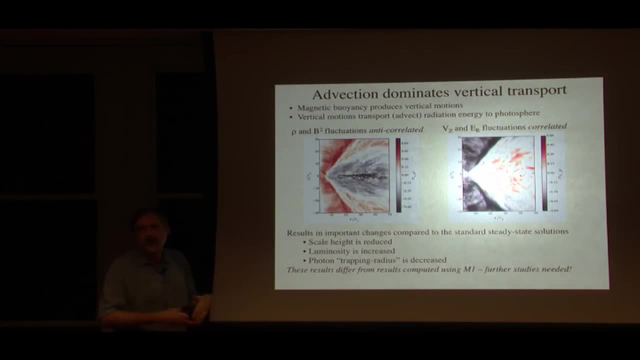 And so that's a very important mechanism which makes the disk a little bit thinner, increases the efficiency and changes the flow, And it's different than the M1 calculations I mentioned before and, for reasons we don't fully understand, It seems to be a generic feature. 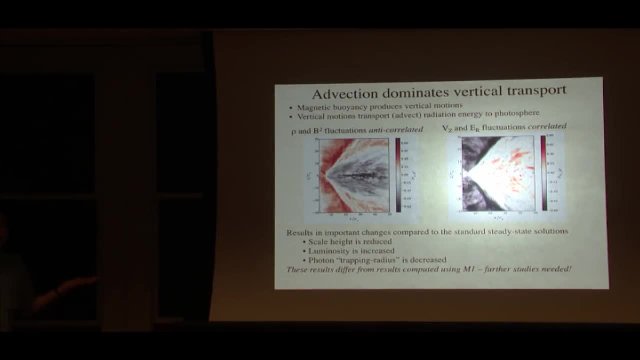 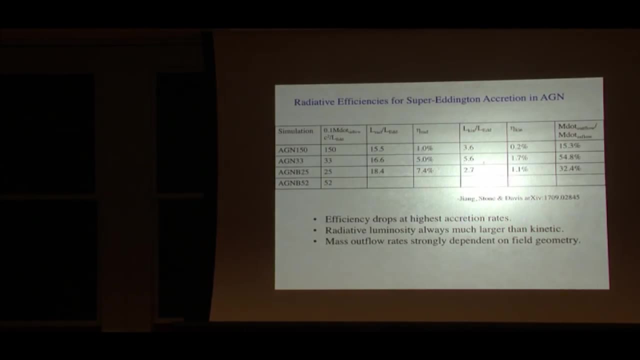 of these MRI unstable turbulent flows. You get this turbulent transport of energy because of these correlations that happen to work out. And so what are those efficiencies We can? for each of these runs, we can measure the mass accretion rate. 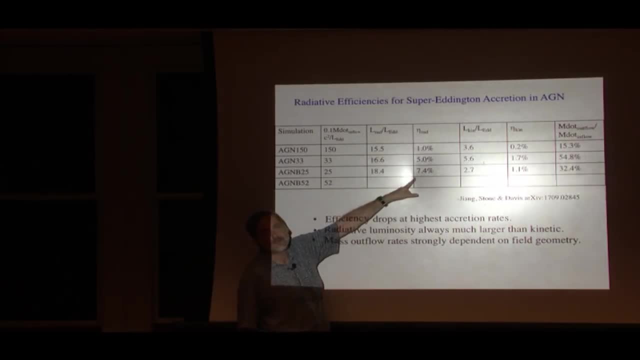 the radiation luminosity at infinity. therefore the radiation efficiency varies between one to seven percent. It drops the higher the mass accretion rate, which is probably good, since you know for very, very high Eddington ratios. it means that the observed luminosity 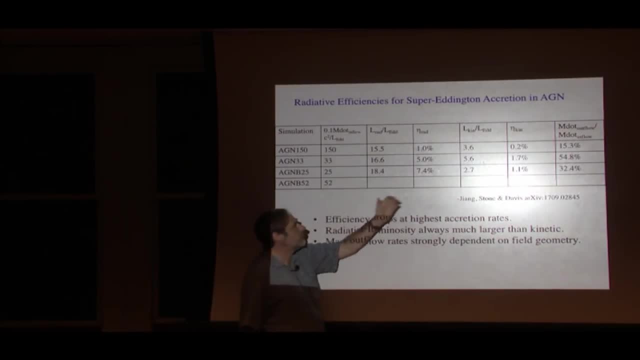 will not be increasing very rapidly. We can also measure the kinetic energy associated with the outflows and winds being driven for this and measure the efficiency of those flows. We can also measure the mass flow significantly less than the radiative efficiency, meaning that radiation feedback 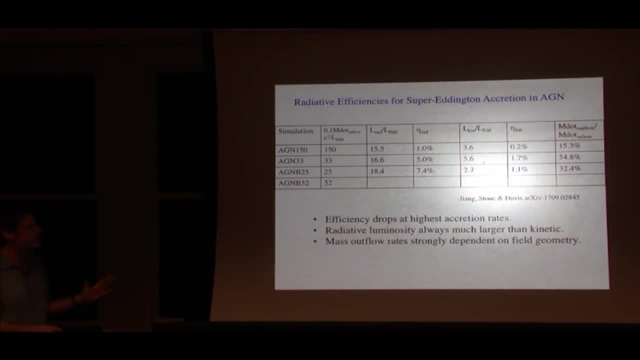 is probably more important than kinetic feedback for this parameter regime here, And we can also measure the fraction of mass flowing out compared to inflow And it's not a uniform. you know dependence on luminosity, It depends on the magnetic field strength as well. 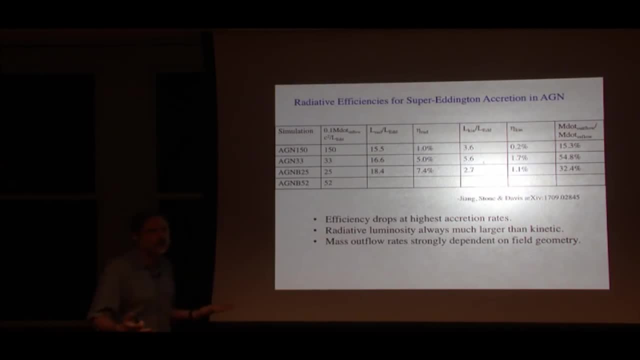 And these models have different magnetic field geometries and strengths, and so there's a magnetically driven component to the wind as well, and that's going to be the outflow rates. So the major points: the efficiency drops at this highest accretion rate. 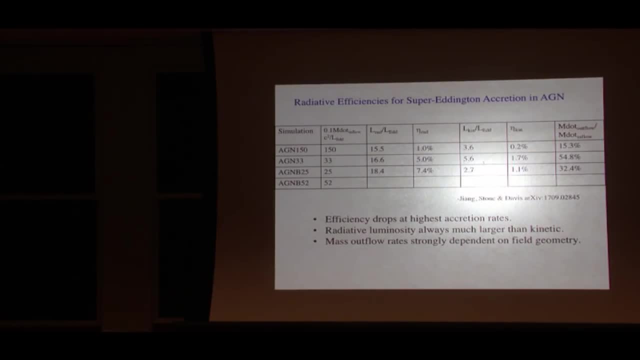 And the rate of luminosity really is the most important thing here in terms of what's going on at large radii. It's going to be the rate of feedback. probably that's important. So what is the difference among the four volumes versus the original radiative field geometries? And the surface density or the surface density. So there's a variety of field geometries and surface densities. The larger the surface density, the larger the mass accretion rate you're going to get. So it's just in the initial conditions. 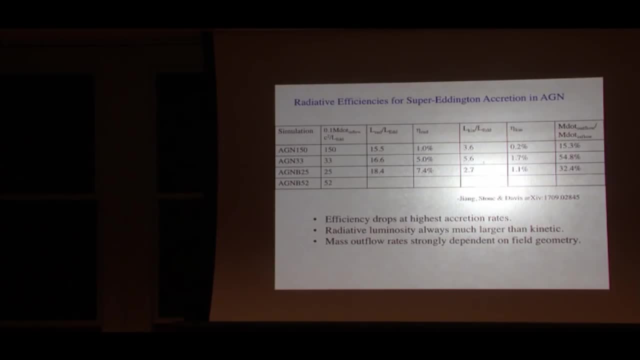 for the torus. that's the only change you can make. There are no net. you know global vertical magnetic fields in any of these models. There is a model where there is a field loop that you know either. the field loops change sign. 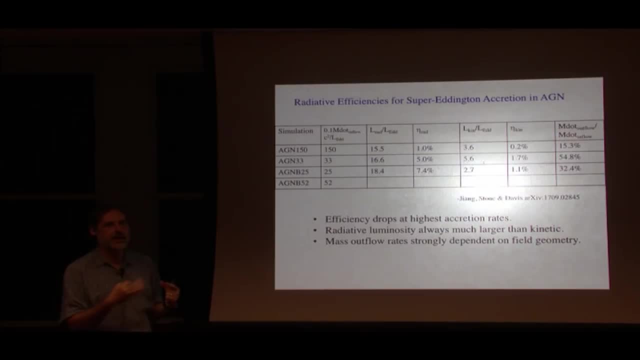 or they don't change sign, And so that generates more net field in patches of the disk than in other patches. So that's why the dynamic of the rainbow layer is so important. I'm sorry, You know. no, I mean, but I don't know. 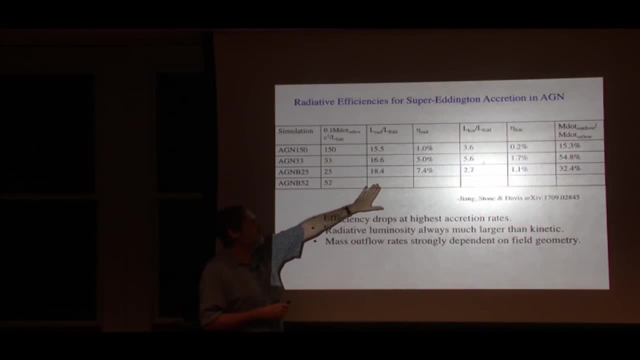 it was shown in the previous slide, but I don't know why the table hasn't yet been filled in. Maybe I deleted it Right? And yes, we've had trouble with the referee. We have a second referee who's very, very supportive. 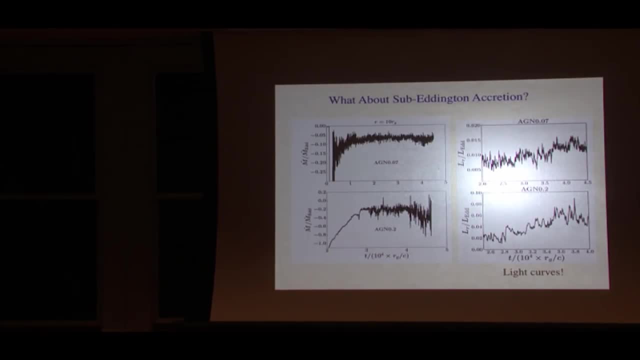 And so? So what about the sub-Eddington disks? By making the surface density much, much lower, you can get sub-Eddington accretion. So here's two models that generate accretion: at 7% of Eddington and 20% of Eddington. 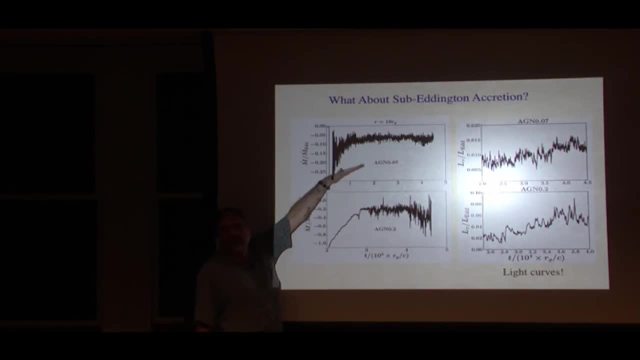 Again they settle down into highly fluctuating but quasi-steady accretion flows And we can again measure the radiative output from them And again, comparing to the Eddington luminosity, these efficiencies are roughly the same you. 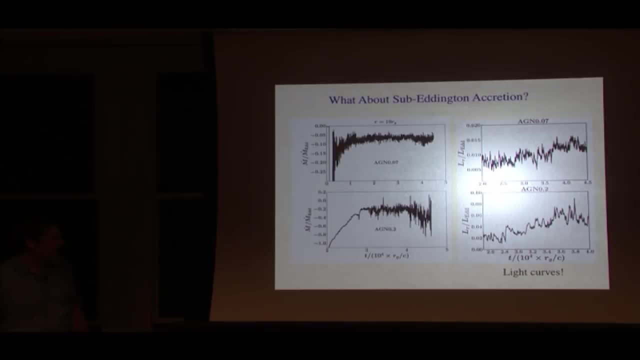 know a few percent to 10% similar efficiencies. I would point out that these are light curves, right? This is what observers measure is how the luminosity is varying versus time, And they're not the same as m dot, which is what people usually use as a proxy for m. 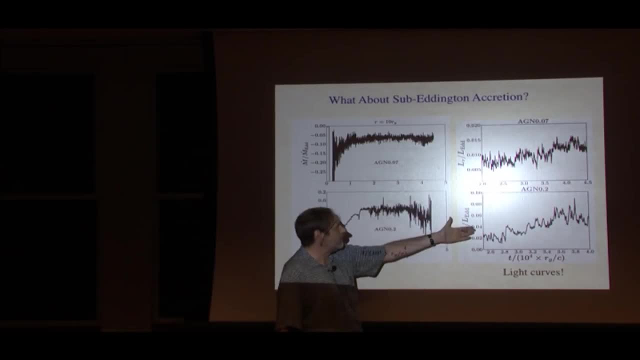 you know what the light variation. So you know there's much to be done in trying to interpret the temporal variability in these light curves, comparing directly to data. There they are, That's the emergent luminosity and infinity. So we can ask you know what does it look like compared to real data? 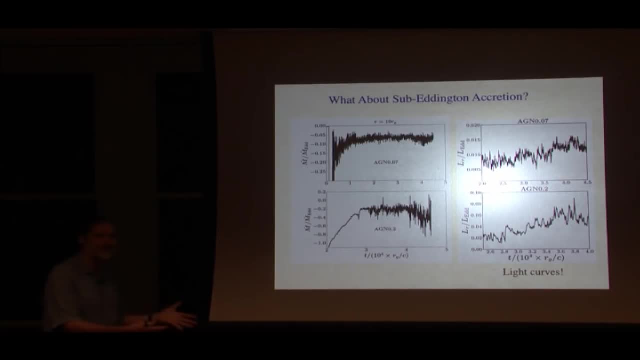 And we can pick that up and again we can do the same thing and then we can get a better picture of it, but for the appropriate bands. And of course this is all for the high energy. you know, this is the very, very center. 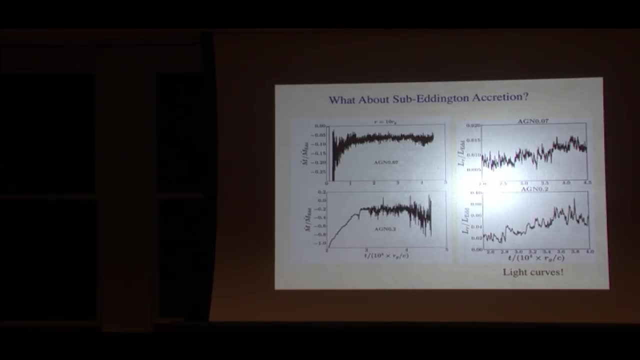 Oh, X-rays, X-rays, soft X-rays probably. Yeah, Quasi-peri—I don't know, You can do FFTs in your eye better than I can. I'm not sure I see anything quasi-periodic there, but yes. 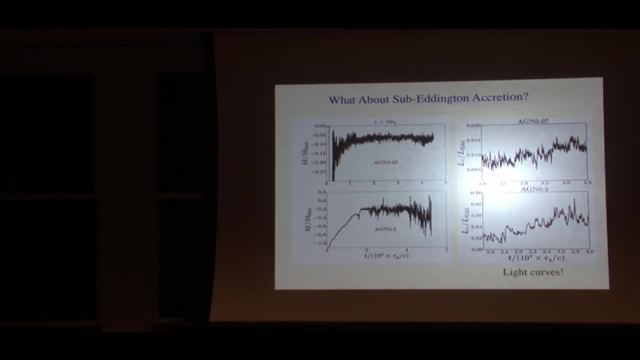 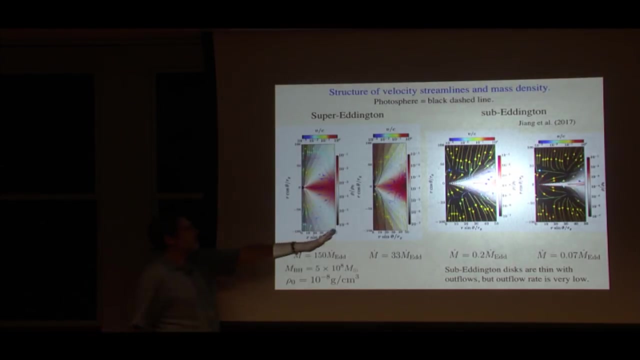 Yes, This is just total luminosity emission. yes, so spectrum is next. And how do all these things compare from super-Eddington to sub-Eddington? So here's four models, from the 150 times Eddington accretion rate down to 7% of Eddington accretion. 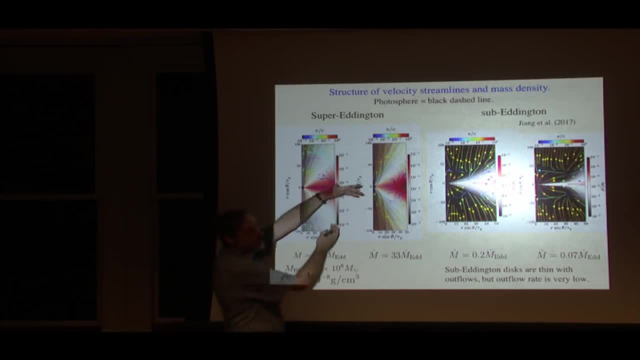 rate. So, generically, as you would expect, the disk gets much, much thinner geometrically as you go to sub-Eddington. These super-Eddington disks are very, very fat and very, very puffed up And there's a lot of material at very high z associated with outflows coming from these. 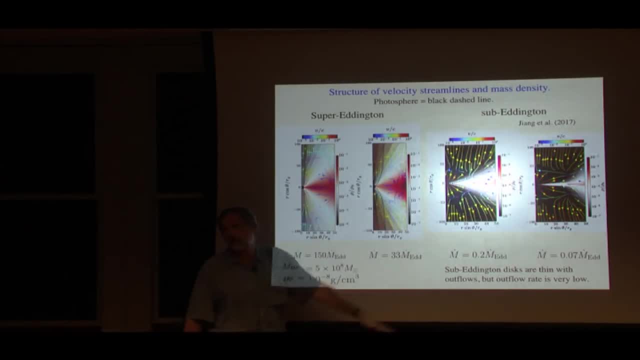 super-Eddington, whereas the sub-Eddington shows almost no outflows, at least from the very inner part, much, much reduced outflows in the very, very inner part. So very thin disks which are still resolved with this nested mesh. 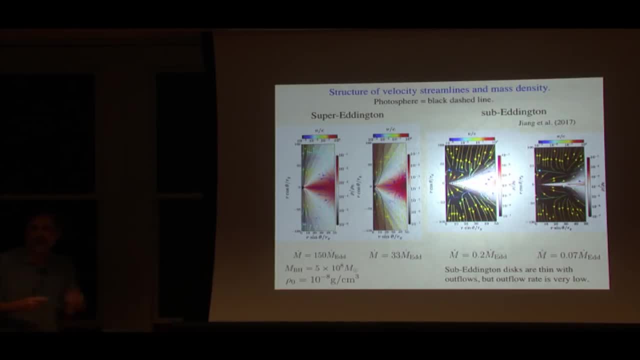 I mean it looks to me that that's That's just a cusp, but in fact if you blow it up, there's still like 30, 40 grid points across the disk thickness there and there's still turbulence and transport going on there. 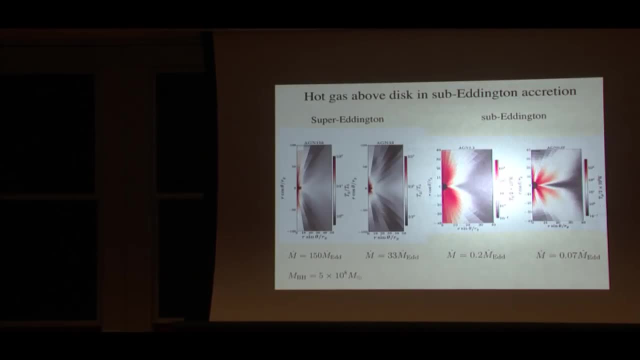 So we see qualitative changes as we change the mass accretion rate. And, getting to Jenny's question, we see very interesting differences in the temperature profiles There's. So these are plots of the azimuthally averaged temperature at various snapshots. for the same, 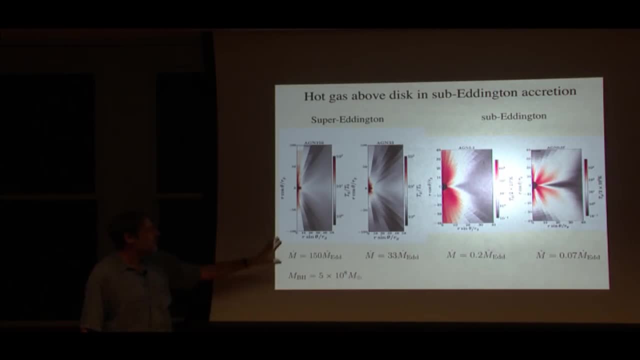 four runs. So you can see the difference between super-Eddington to sub-Eddington. And what's most interesting is in the sub-Eddington case you begin to see the emergence of very, very hot gas in the polar regions and then eventually, over a significant range- 20 to. 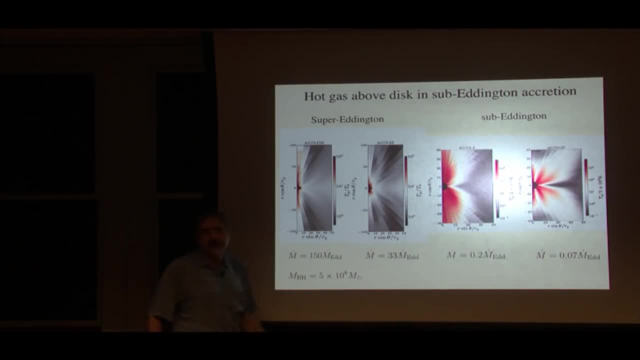 25 Rg, a few scale heights above the surface of the disk, there's this very, very hot gas appearing in the flow. So that's very interesting. We'll return to that in a minute. But some other basic properties of these accretion flows: 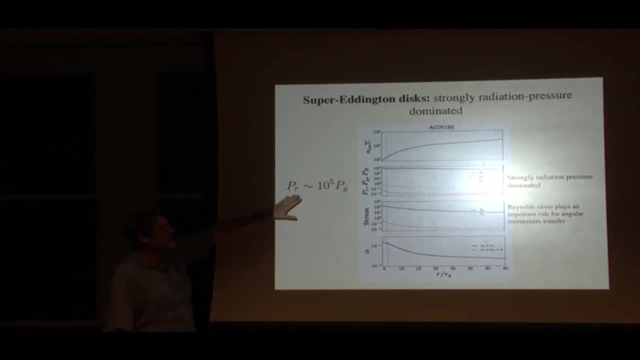 These super-Eddington disks really are strongly radiation pressure dominated. So these are now radial profiles of azimuthally and time averaged properties in the disk. So, for example, the opacity or, sorry, the optical depth is enormous, up to 10 to the. 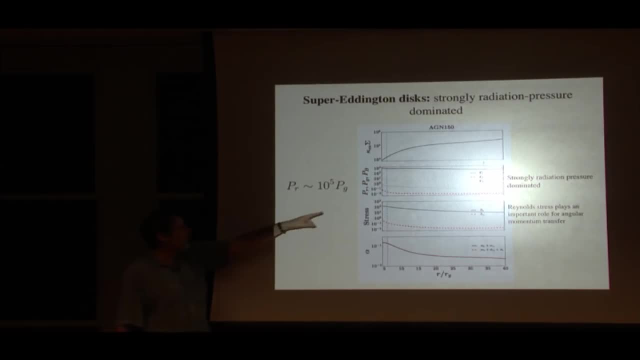 5 across the disk as a function of radius. But interestingly, the radiation pressure, the black line, compared to the gas pressure, this dotted line, is enormously different. There's a ratio of 10 to 5.. Yeah, 10 to the 5.. 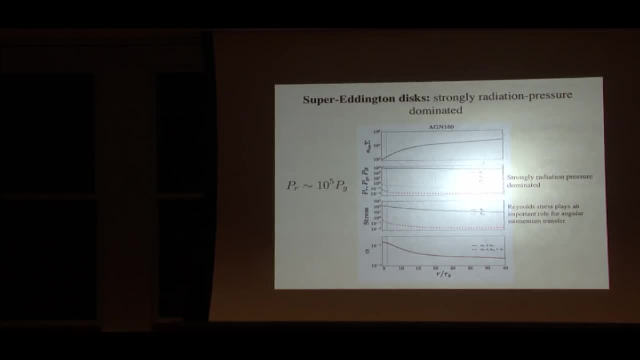 So in these super-Eddington regimes, these really are radiation pressure dominated, where, for example, the radiation damping is playing a big role in the MRI, And that means that it seems the Maxwell stress in this case is significantly smaller than 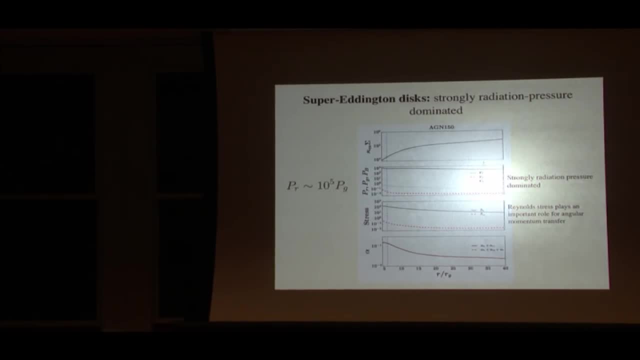 the Reynolds stress. The Reynolds stress is associated with these spiral modes that I showed you before. So there's this one regime of very strongly radiation pressure dominated appears in the super-Eddington. In the sub-Eddington case you don't see such a big difference. 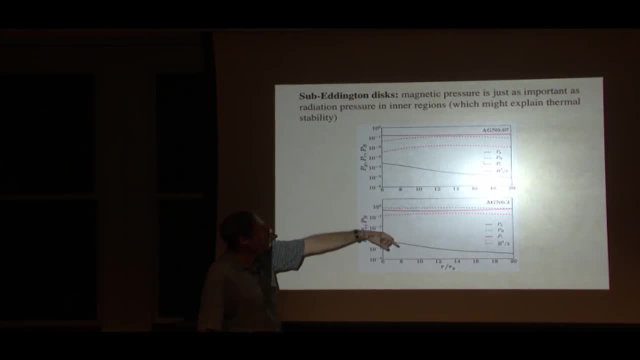 Well, the radiation pressure and magnetic pressure are not that much different. So the radiation pressure is the red line and the magnetic pressure is the black dashed line, And now they're within sort of 10% or even larger compared to the two. 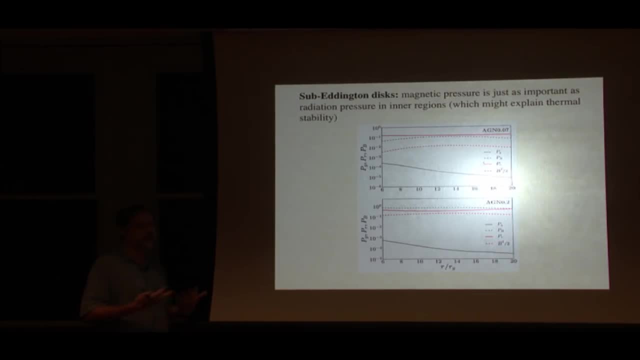 So in this case magnetic pressure is playing a role in the structure of the disk. In fact, I said that radiation-dominated disks are thermally unstable. in these shearing box calculations They show thermal runaways. Yeah, So you don't see any evidence for thermal runaways in these sub-Eddington global calculations. 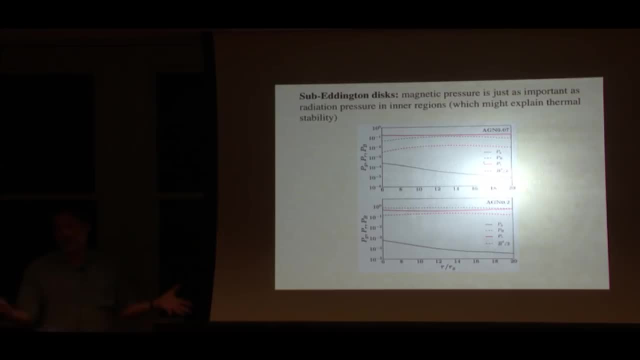 even though they've been run for many, many hundreds of orbits, many thousands of orbits in the inner regions and many thermal times. And one simple reason is that perhaps this magnetic field is playing a significant role in the support, Because the classical analysis is for gas pressure-supported disks with magnetic pressure. 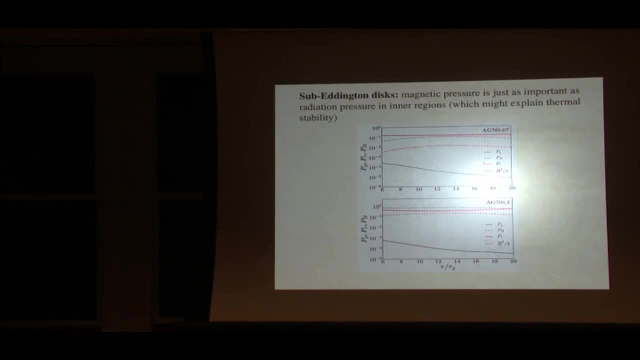 It wouldn't be surprising if the stability properties of the disk were quite different. So that may be one explanation. Yes, That's correct. Yes, We don't get as much magnetic pressure in those calculations as you do in the global calculations. 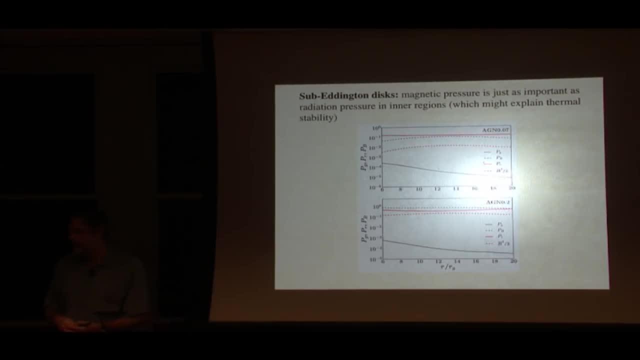 They are a slightly different parameter regime. It is true that in the coronal regions of the stratified disks you do see very, very strong magnetic pressure, but not towards the mid-plane like you are here. So they are a little bit different than the shearing box calculations. … It appears later. 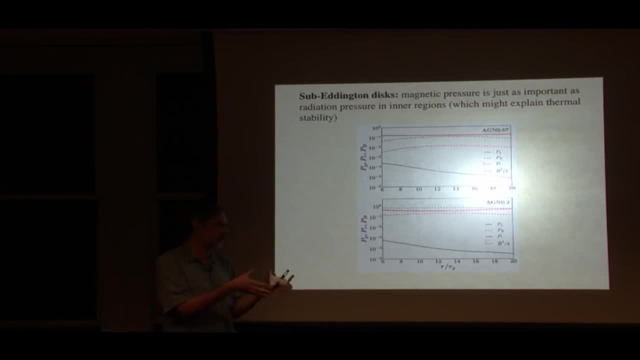 Integrated over the entire box, there is no mean field. But if you take some region, say the inner 10 shorter radii, you can generate a mean field there which is connected to the equal and opposite field at the larger radii. 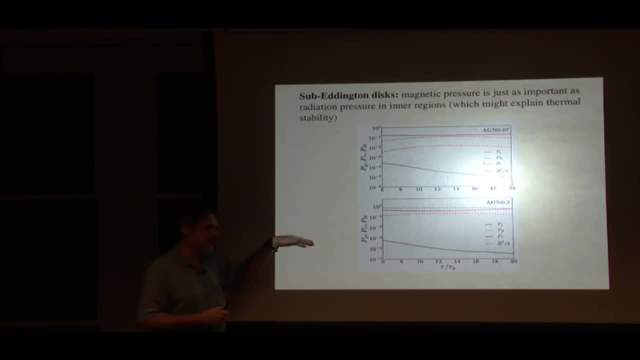 We actually haven't really studied or plotted the mean field versus radius to know what it really looks like, whether or not we really do see mean fields preferentially in the regions. that's. that's a good diagnostic. we should look at some more, that's correct. 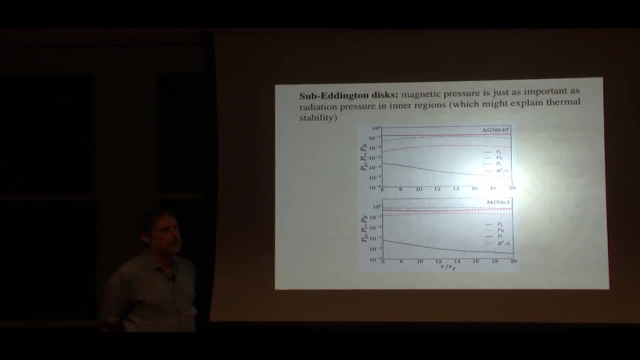 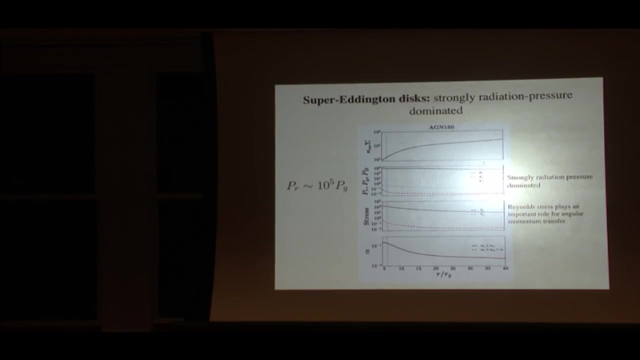 that's correct. yes, you know, once it's reached steady state and saturated, the fields become readily constant, steady in time. that's when those modes are most important. yep, yep, it's Reynolds versus Maxwell stress, so it's a huge difference. yep, that's right. 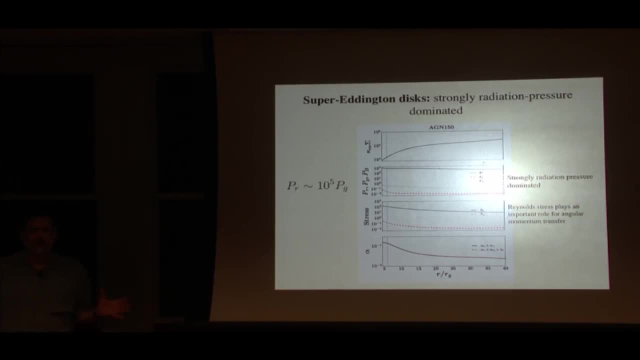 you know it's not. I mean it's weird because if you take the magnetic field away, there's no turbulence, there's no spiral modes, there's no Reynolds stress. you put the magnetic field in, it generates turbulence and waves. they get amplified. you get these spiral modes, you get this Reynolds. 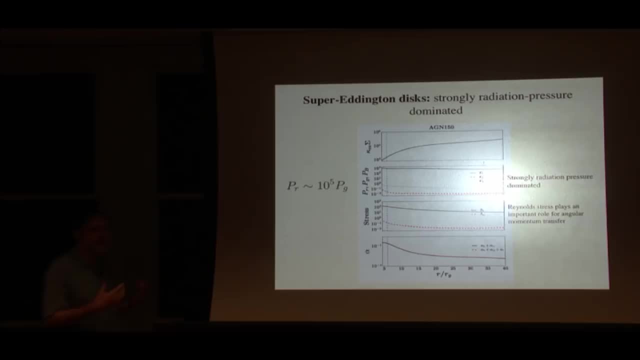 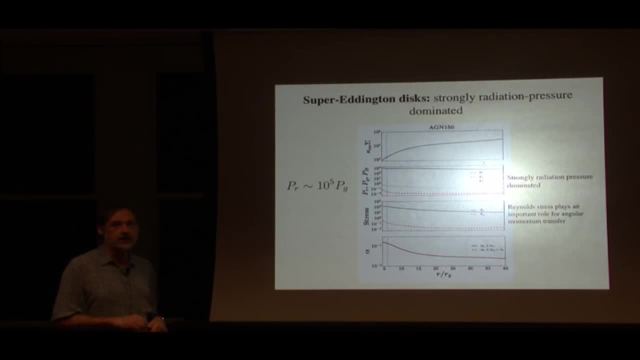 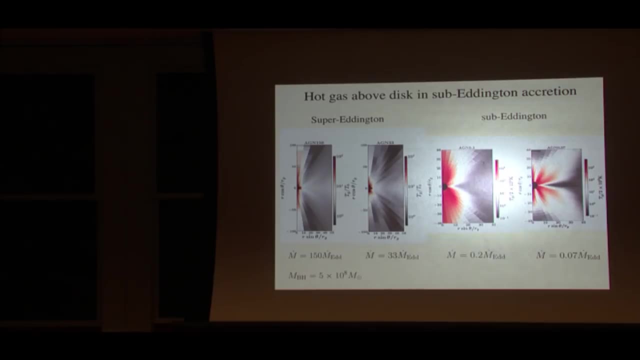 No, No, Definitely not. You know, you do these calculations with, say, a gamma four-thirds. you don't see these spiral modes. You really need to compress a bit So strongly radiation pressure. one of the most important features is that it's extremely highly compressible. 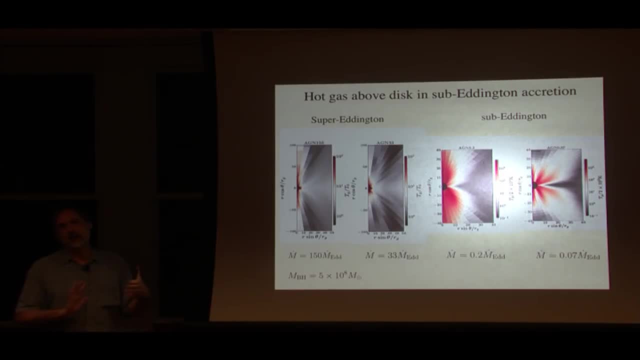 because the radiation can leak out as you start compressing it, and you know the radiation pressure is enormous, And so you compress, compress, compress, compress until finally you get to gas temperatures that can resist it. So this was seen long before that these flows are really, really, really compressible. 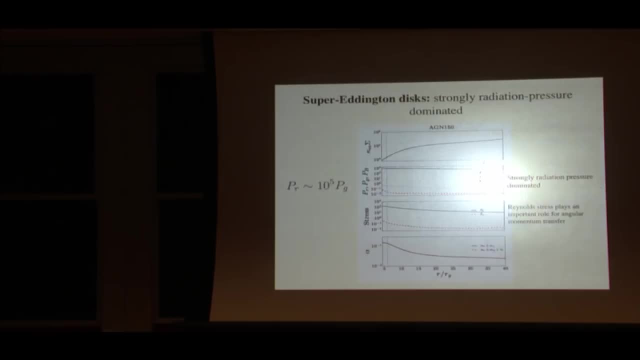 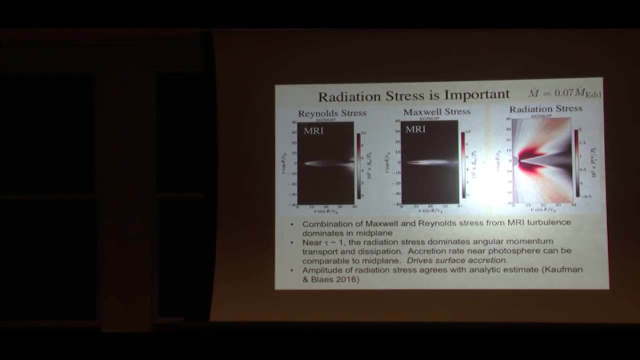 and that's probably my guess- playing a role. Okay, So those were the sub-Eddington disks. Actually, it turns out that radiation stress in these sub-Eddington disks is important. So here is the- again time and as mutually averaged colloidal plots of the stress. 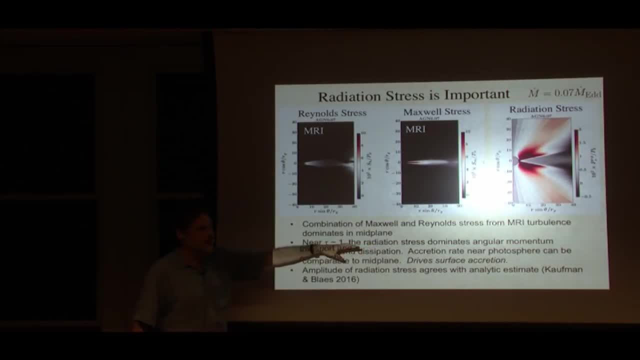 the Reynolds stress, the Maxwell stress and the radiation stress I mean. after all, there is a radiation pressure tensor whose R-phi component is the angular momentum transport rate due to the radiation field. So that's what that last plot shows you. 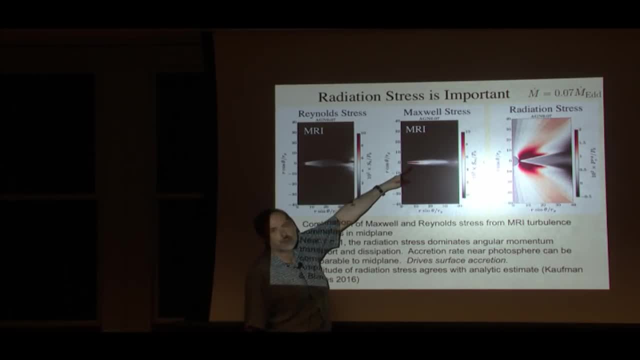 So you see the classical MRI producing Maxwell stress in the disk mid-plane, which then produces Reynolds stress associated with the turbulence. The Reynolds stress is smaller than the Maxwell stress as the standard MRI picture. But what's interesting is that above the mid-plane, not in the middle where the MRI dominates. 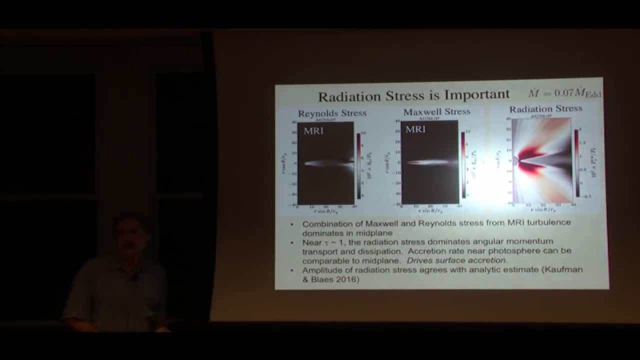 but above the mid-plane you begin to see significant radiation stress. That's where the photon mean-free path is starting to get large. It's the optical depth one. You need a large mean-free path to get you know angular momentum transport due to the photons. 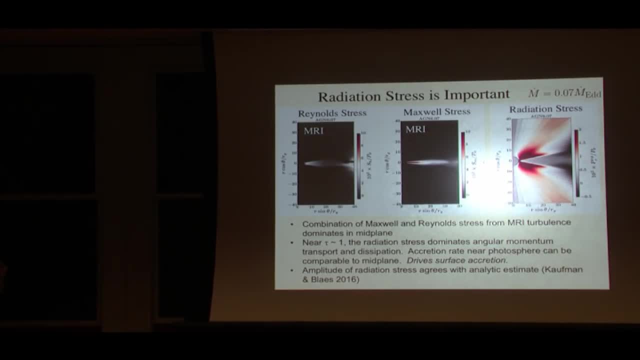 That's exactly where it's happening. In fact, it drives this surface Surface accretion layer. The angular momentum transport due to the radiation field is driving some accretion at the upper layers. It's smaller than the MRI stress integrated over the volume, but it's non-negligible. 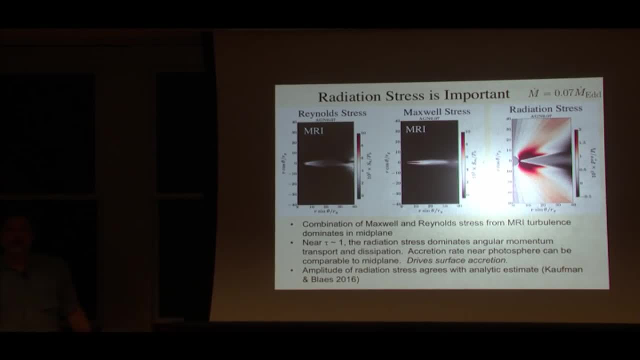 Interestingly, it agrees with analytic estimates for what that stress should be for these parameters, which is also very reassuring, And again, it's something you couldn't capture without this full transport algorithm. If you make some approximation about the closure, you're never going to get this radiation stress tensor correct. 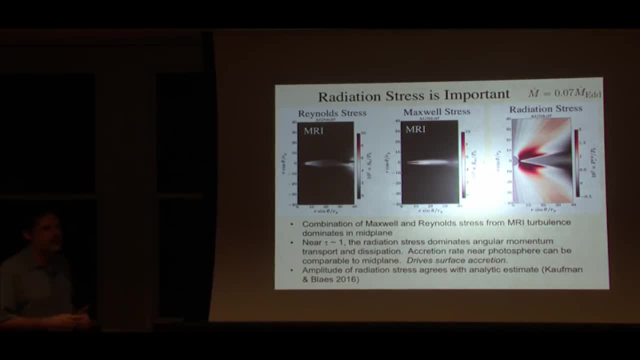 because you're going to assume what it is, not compute what it is. So this radiation viscosity effect only comes out when you do the full transport. Yes, We have not done that experiment to repeat this calculation with M1. And that would be very, very useful. 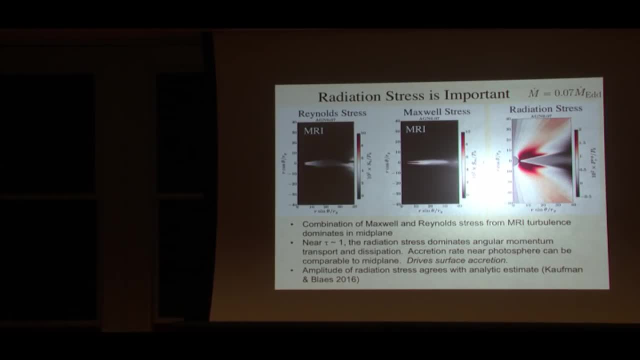 However, with M1, you wouldn't get that radiation stress, So I think it would have to be qualitatively different. It seems no, This is mostly important in the sub-Eddington and mostly in the upper layers, And again, these upper layers get really, really hot. 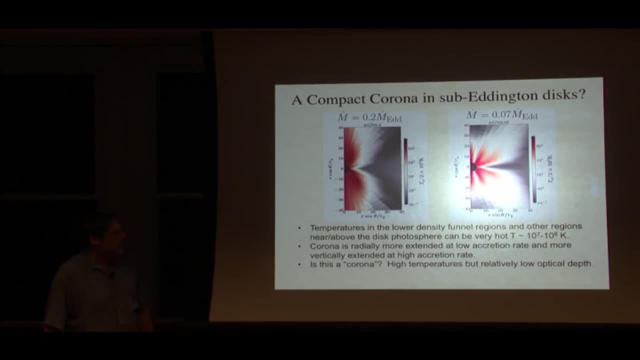 And here's the 20% and 7% of Eddington. Temperature is 10 to the 7 to 10 to the 8 Kelvin above the disk mid-plane. So is this a corona? It turns out that the surface or the optical depth through this hot gas is pretty low. 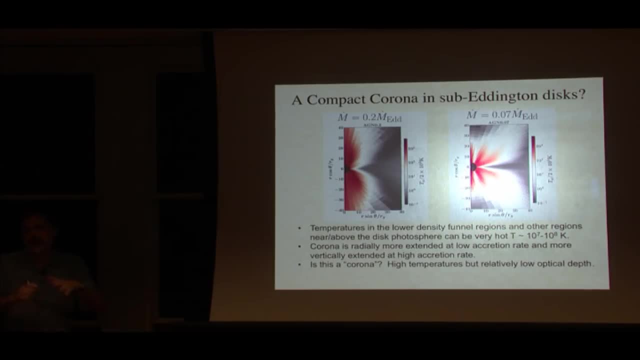 And so when you compute spectra of these, you do get a nice soft X-ray, But the ratio to that, to the optical bump, is still not high enough. We're about- I don't know, we're about a factor of 3 or 4 below where we should be. 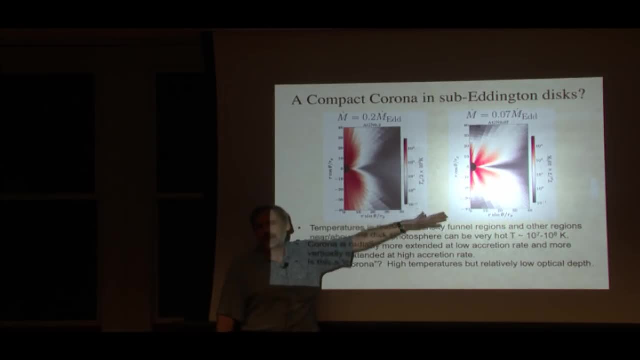 But interestingly we get this broad extended soft ray excess just from a multi-temperature hot gas above the mid-plane which has emerged self-consistently from MRI plus radiation transport, And that's kind of interesting. So we're trying to do more with M1.. 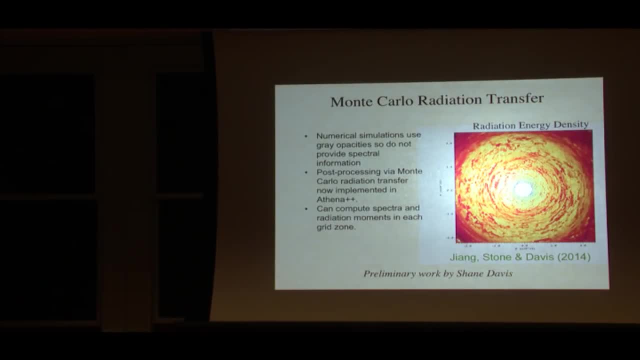 We're modeling spectra, And so Shane Davis has implemented a Monte Carlo radiative transfer which can be used to post-process the results. We're using these ray methods for doing the dynamics, but they're based on continuum capacities, And to model the spectra we're post-processing the data with Monte Carlo. 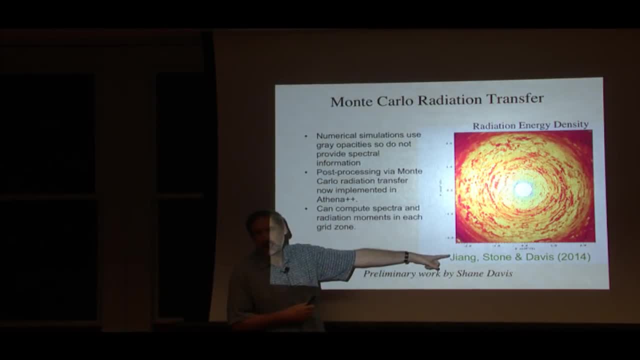 So, for example, Shane takes a snapshot from one of the 3D disk calculations and calculates the radiation energy density from the Monte Carlo And makes sure that in an averaged, in a volume average sense the profiles agree exactly with the sort of consistency check. 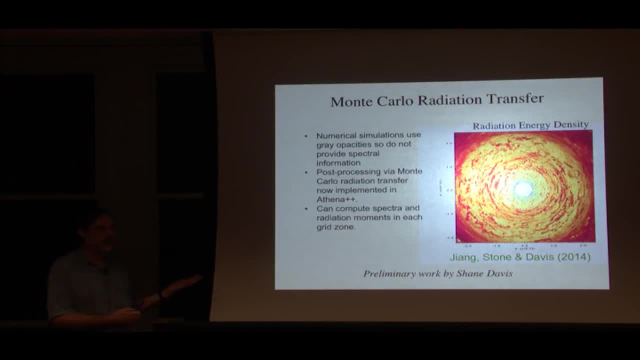 to make sure that Monte Carlo is giving us the same radiation, energy density and flux as what the dynamical code is giving us? Question: Yes, We do include proximate treatment of Comptonization in the upper layers And Shane's calculation, I think, includes it completely. 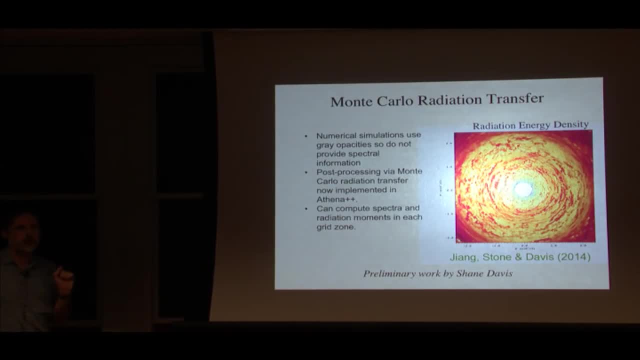 So it's only this continuum electron scattering plus. yeah, Our biggest weakness is in the way we treat the high energy process like Compton scattering. So we just calculate gas temperature differences compared to some fiducial temperature difference and we use that to estimate what the Compton rates are. 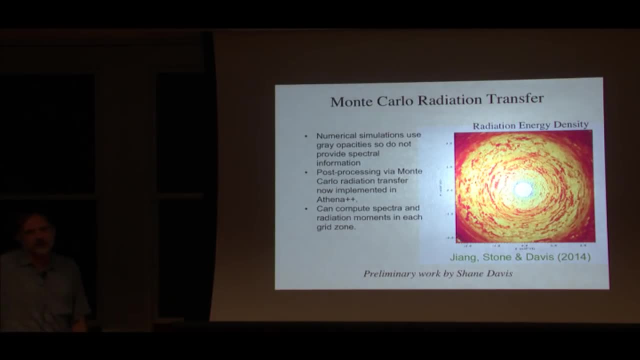 And that's Compton. cooling is a specifically difficult thing to do ab initio And it's going to remain some work to get it done exactly right. One reason I want to show this picture is because Monte Carlo looks like a very attractive way. 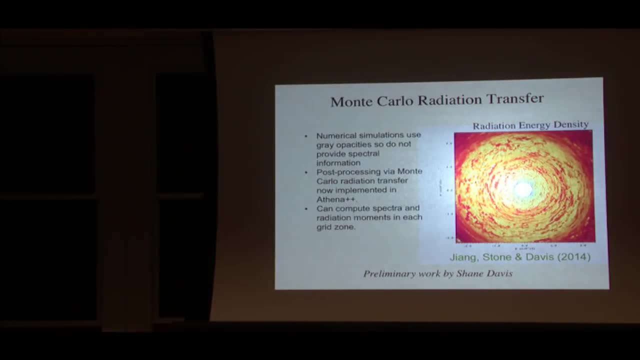 of doing radiation transport in the future as well, except notice the Poisson noise you get from Monte Carlo. This is the radiation energy density, with still, you know, 10, 20% fluctuations And this will do violence to the dynamics when you're in a radiation pressure dominated regime. 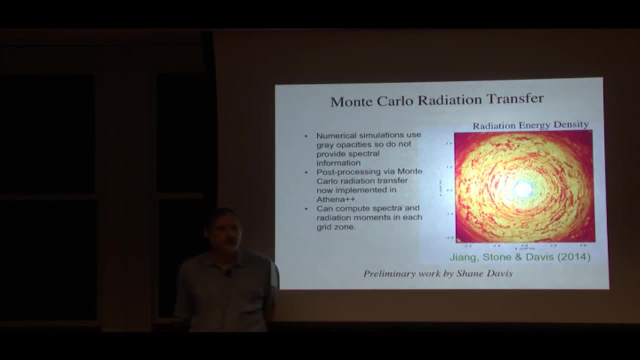 You can't allow 10 to 20% pressure fluctuations from cell to cell And to beat that down. I mean, how small do you need it? 1%, .1%. that's going to take, you know, an enormous number of photon packets in each cell to get that in. 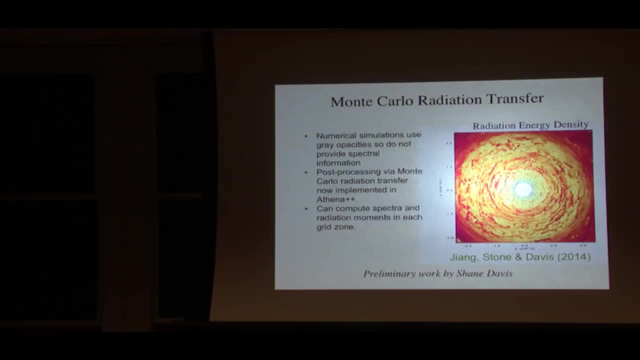 So that's the only challenge of using Monte Carlo is getting the Poisson noise down. Sort of the same issue with PIC versus continuum approaches. It's all about the noise and the cell to cell noise. So of course I'm going to cherry pick the best spectrum that we've been able to compute so far. 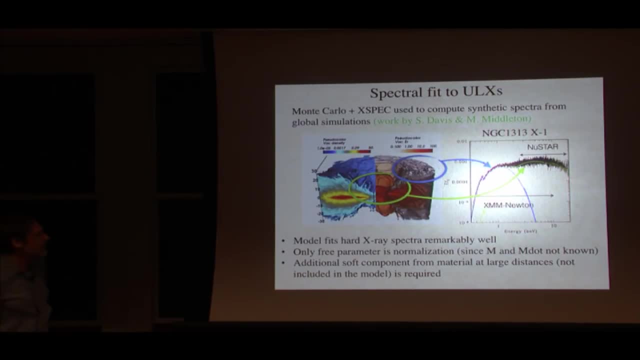 Shane Davis and Matt Middleton have compared the spectra computed from their Monte Carlo solver, which they then feed into X-Spec to get the instrumental response correct, And then they compare that directly with XMM and NuSTAR data for a particular ULX source listed here. 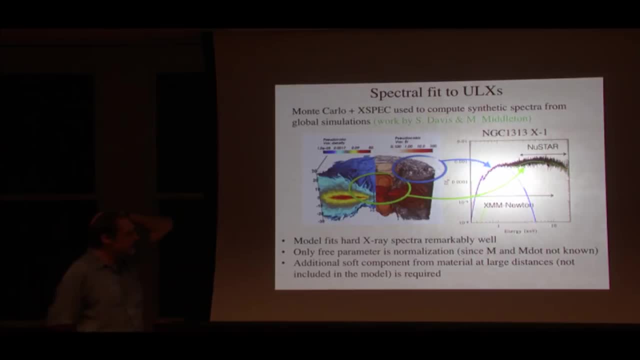 The wiggly line is, of course, the data, And the blue and the green line are portions of the fit that come from various parts of the spectrum. This is the simulation domain And you can see that the fit is pretty good, especially in the high energy, this very, very broad high energy tail. 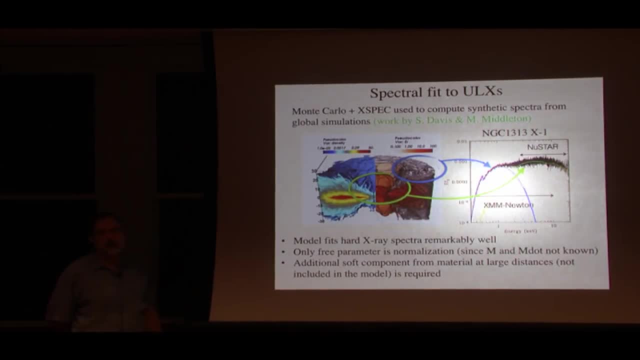 What would be the soft X-ray excess in AGN is fit remarkably well And it's just simply coming from this very, very multi-temperature hot gas, very hot, multi-temperature gas in the inner regions. There really isn't any parameter fitting here, except we don't know the normalization. 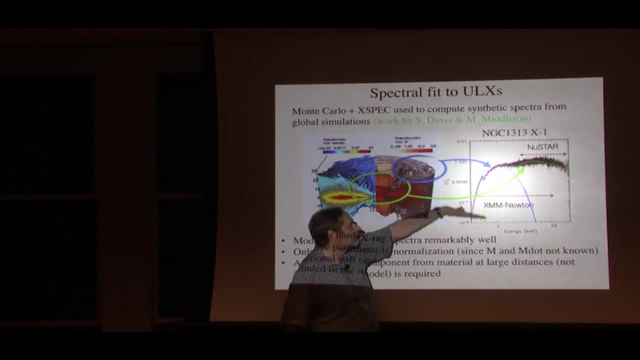 We don't know the mass of the black hole, We don't know the secretion rate. So you can slide this curve up and down. The total flux is unknown, But you can't change the shape of it. That's determined by the distribution of optical depths and temperatures that come from the calculation directly. 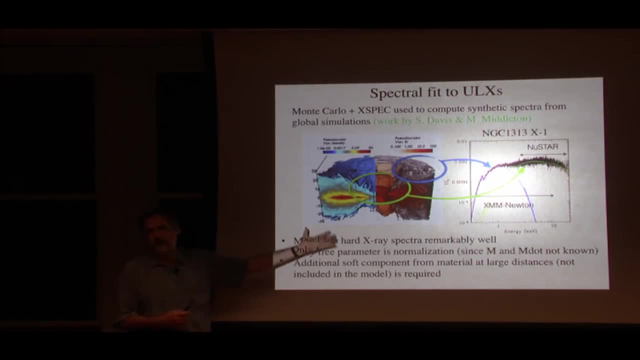 So I think this is very, very encouraging. You know, the fits to the AGN are not nearly as good, and we're working on understanding why that is in the future. Okay, so let me wrap up with where we're going in the future. 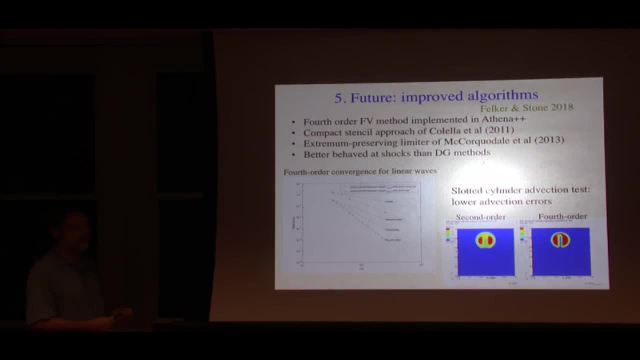 So one thing is to improve our network, One thing is to improve our numerical algorithms- Always important to improve our algorithms- And Kyle Falker has implemented this new fourth order transport algorithm in Athena++. It greatly reduces advection errors. Here's an advection test between second order and fourth order. 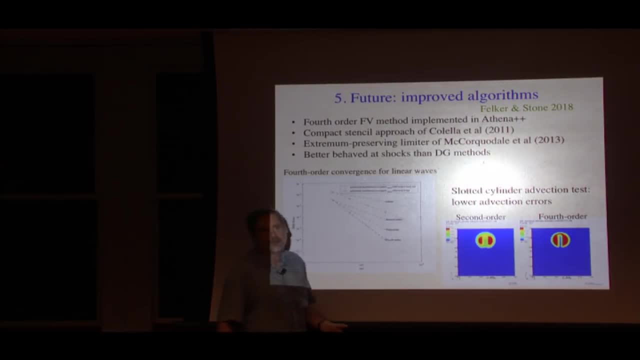 A slotted cylinder which is only five cells across And you can see it captures it even after advecting around the circle a couple of times. It does extremely, extremely well. There's a lot of interest in moving mesh methods to reduce advection errors. 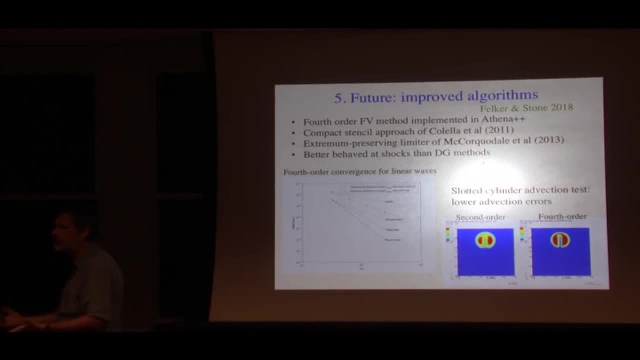 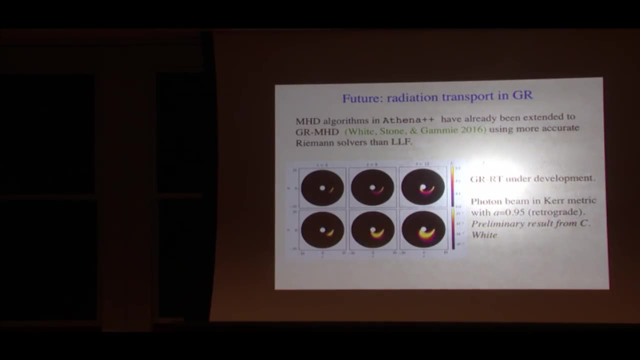 It seems to me that these higher order methods look just as attractive and have all the advantages of finite volume methods, And so we're pursuing these to improve our calculations, And we're also trying to do the full GR. Chris White had already implemented full GR for the dynamics. 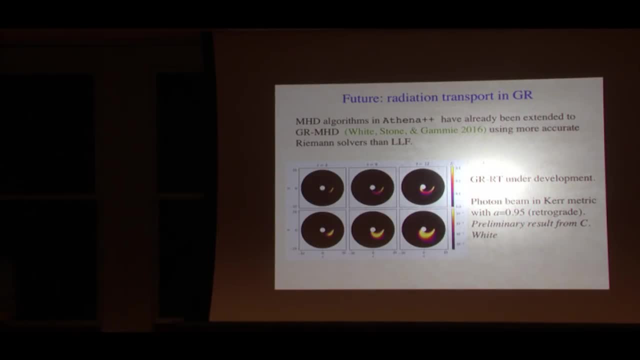 What we don't have is full GR for the radiation transport, Because doing these ray tracing methods in full GR is much more complicated than doing M1 or FLD in full GR. But recently Chris White has been prototyping a method in two dimensions. 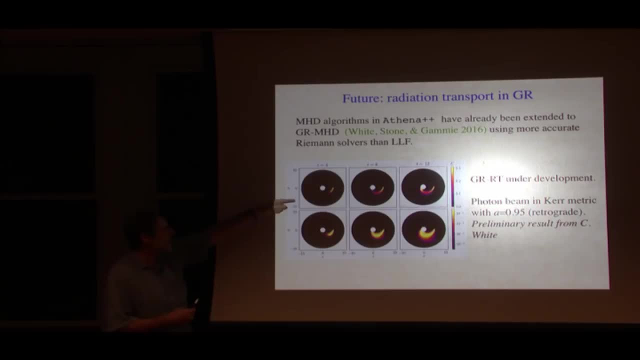 Which looks very attractive. This is the transport of radiation in an optically thin beam In a stationary space time for a care metric with retrograde spin 0.95.. The dashed green lines here you can't see in the back, I'm sure. 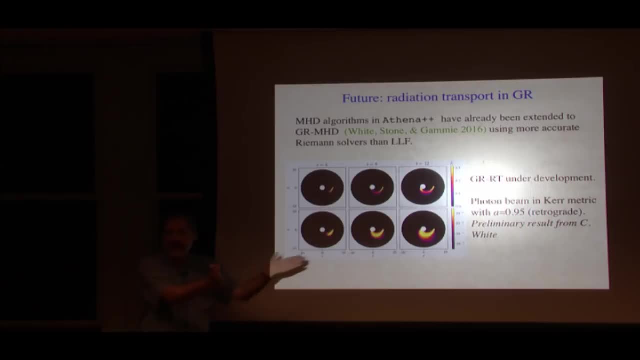 That is the cone which this flashlight beam is supposed to be spreading out over, And you can see that the numerical solution is following these geodesics extremely well, And so our hope is to implement this in full three dimensions And then migrate at the full dynamical code. 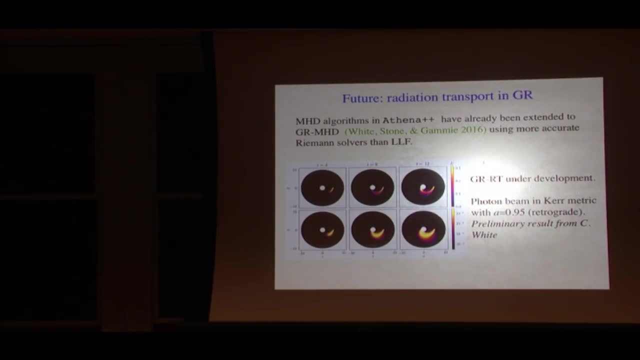 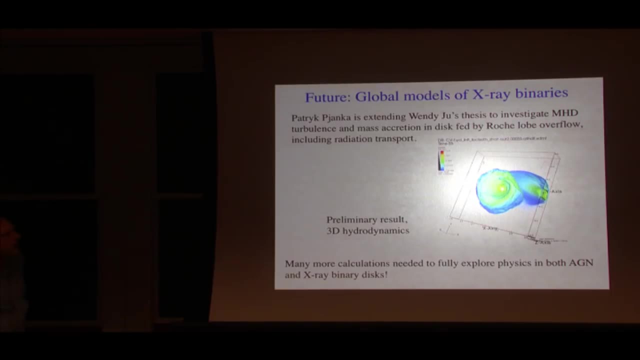 So we can truly study black hole accretion flows, including at the middle with spinning black holes. And then finally, Patrick Bianca is also looking at X-ray binaries And mass accretion and properties of radiation. dominant accretion flows in close binaries.